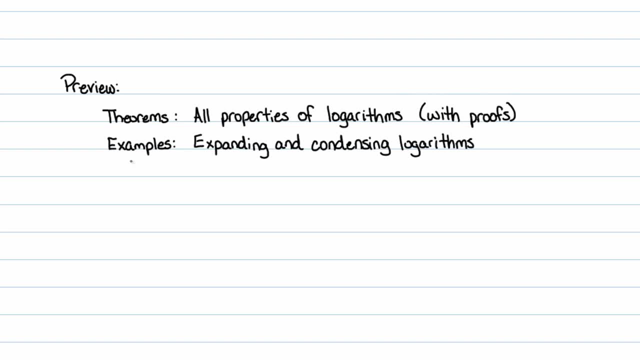 with proofs, as I said a moment ago, and the examples. We're going to have a bunch of examples on expanding and condensing logarithms. Other examples, like applications and stuff like that, will be saved for the next lecture. The prerequisites required for this lecture from you. you have to know all stuff about. 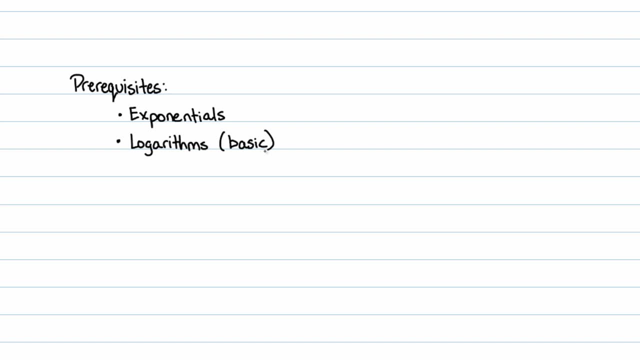 exponentials, exponential functions, how to convert between exponential form and logarithmic form, and you should know the basic stuff about logarithms. what a logarithm is that type of thing? Now recall that if b is not equal to 1 and is positive, then b to the y power is equal to x. 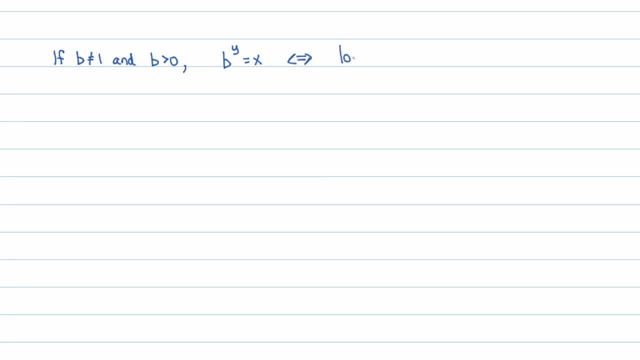 is the same thing as saying log base, the same base as that exponential of x is equal to y. And again this, I always kind of refer to this, getting back between logarithmic and exponential form, as doing the circular argument, b to the y power is equal to the inside, which is x. 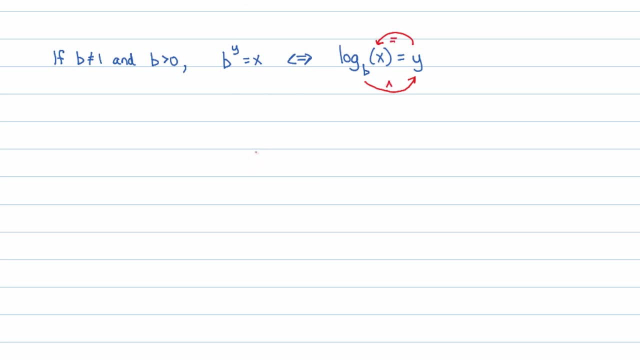 That's how I would transform between these two forms easily, Just without having to memorize too much. Also, it is assumed, because x is equal to some exponential function where the base is positive, that x is positive as well. So just letting you know that this means that x must be positive because it's equal to a. 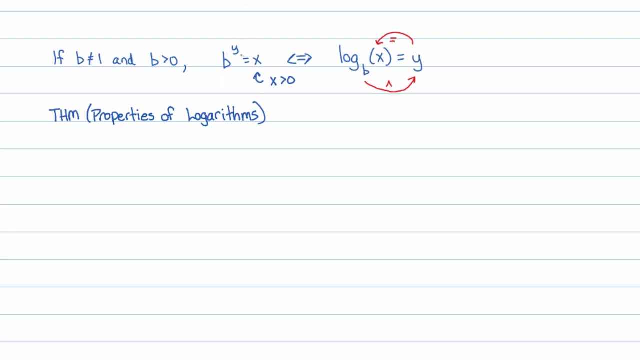 positive number raised to any power. Well, positive number raised to any power is going to be positive. Okay, now let's go into the properties of logarithms here, and I'm going to write down the few basic ones that we've talked about already. The first one, and each of these I do not want you to memorize, I'd rather you really just 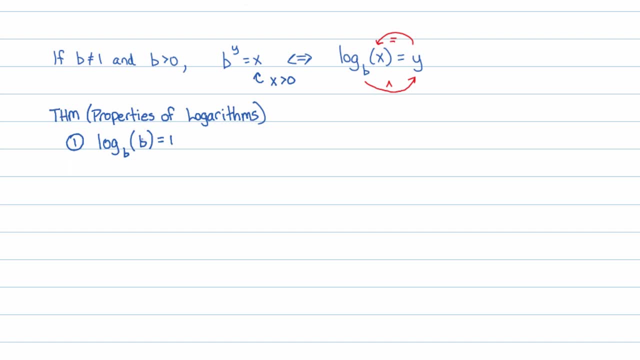 try to understand this. The first one is that log base b of b is equal to 1, and the reason why this is true is because, well, using a circular argument, b to the first power- maybe I'll use red instead- b to the first power is equal to b. 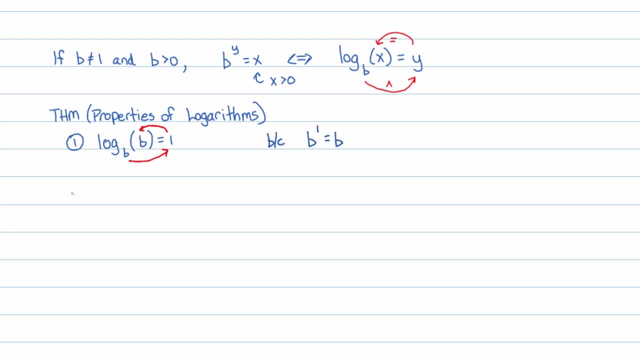 So I'll write that over here. The second property is really kind of an extension of this property here. So log base b of b to the p power is equal to p, and that is because, well, if you use a circular argument again, b raised to the p power is equal to b to the p power. 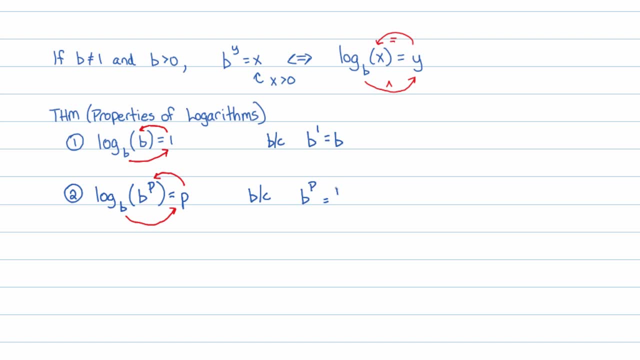 So I'll write that down: b to the p power is equal to: well, b to the p power. that makes sense. Okay, The next property we discuss is log base b of 1.. Well, log base b of 1 is equal to some number. let's see b to what number is equal to 1.. 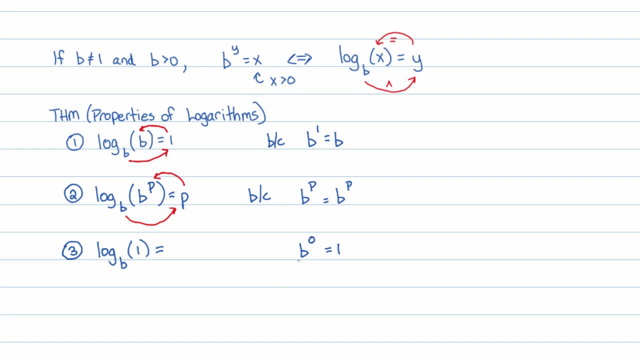 Well, b to the 0th is always equal to 1, especially because b is positive. So b to the 0th, power is equal to 1.. Using a circular argument, you can see: b to the 0th is equal to the inside, which is 1.. 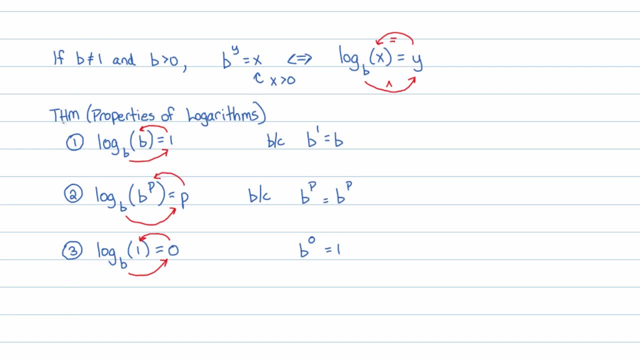 The one that I proved in the previous lecture- Let me do this in the right color- is the following: b raised to the log base. b of x is equal to x. I forgot to write that because in there, and the reason why this is true is well, you kind. 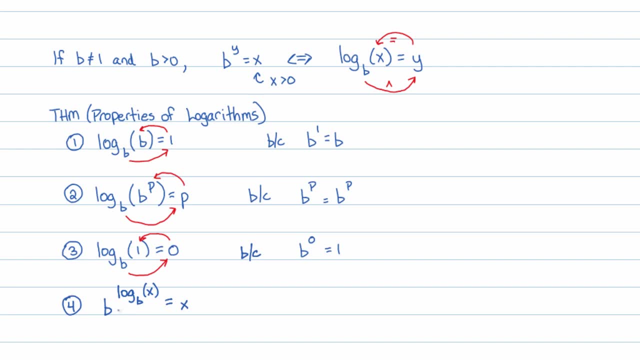 of just use the circular argument here, but in reverse. Now, if you look at this example or not, the example- Not the example, but definition of a logarithm up top b to the y power is equal to x, truly implies is the same thing as saying that log base b of x is equal to the exponent. 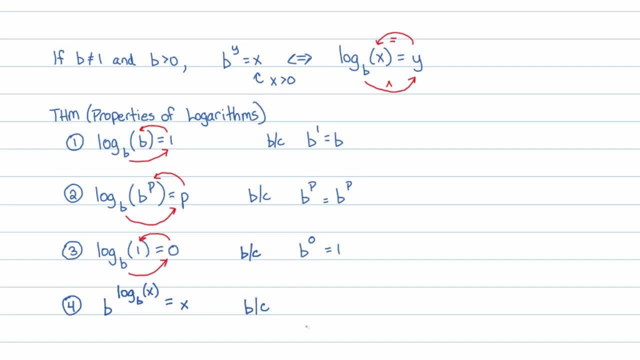 So this is true because log well, the base of this exponent is b, So log base that b of x is equal to the exponent, and the exponent here is log base b of x. Okay, And that's that's why that's true. I mean it's. there's not very much else I could say about that one, that's just true. and you. 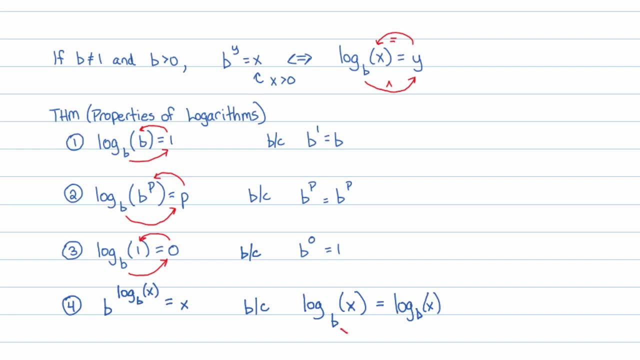 could use the circular argument to see that is true. B raised to this picture is equal to x. B raised to log base b of x, which is right here, let me highlight it right here- is equal to x. So I guess that must be true then. 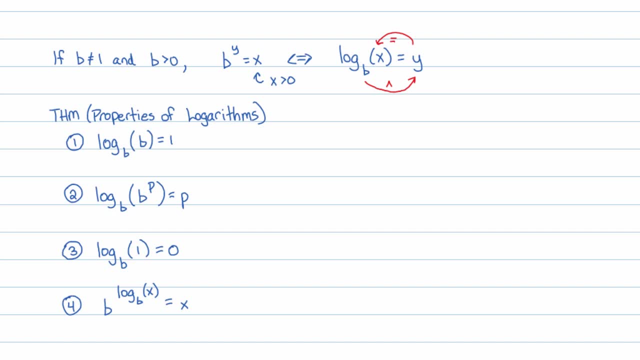 Now, Those are our first four. there are actually a few more that we're going to go through in this lecture, and I'm going to prove each one of them. The fifth one is log base b of m times n. I'll just use those two letters. it could be any two letters I want, as long as those two. 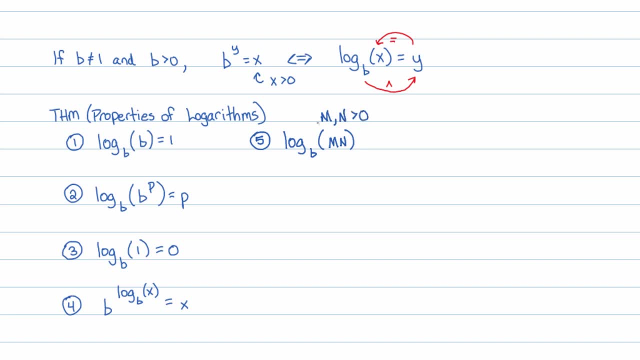 letters m and n are positive. Okay, And remember, whatever goes inside a logarithm has to be positive because remember, by definition, What's inside the logarithm here is what was equal to the exponential function, and remember exponential functions are always positive. So you need the inside of your logarithm to be positive. 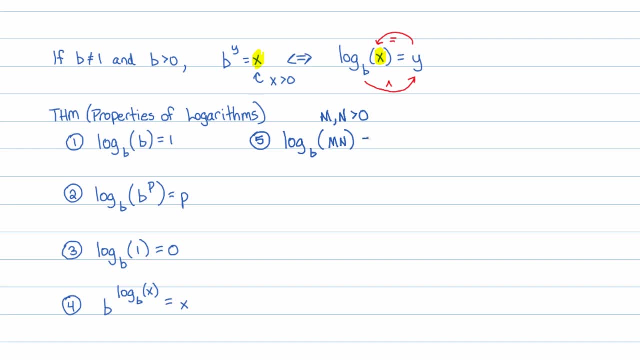 All right, so log base b of m times n is equal to log base b of m plus log base b of n. We're going to prove it in a moment. Actually, I might as well prove it right now. Okay, So here we go. 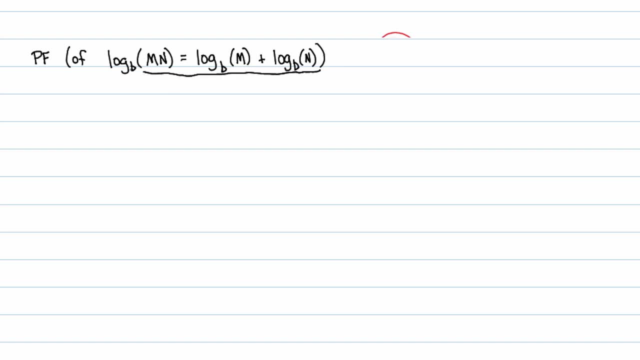 The proof of this property here. First thing I want to draw your attention to- and this is not part of the proof, but this is very similar to the following property for exponentials that x raised to the m power times x raised to the n power. so notice, I'm multiplying these two exponential functions. 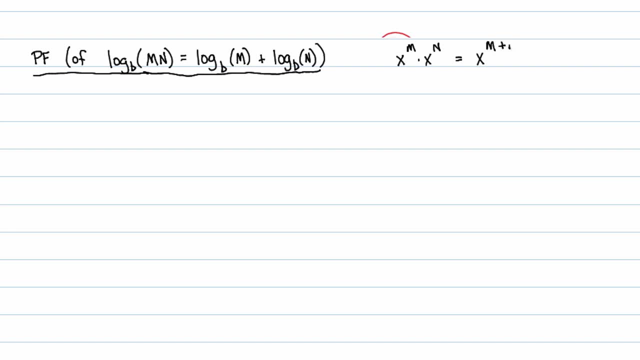 is equal to x, to the m plus n. notice: when I multiply them together we get an addition. notice here with logarithms: when you multiply insides together you get an addition. so this is very similar. it stems from this property. that's not part of the proof, but I'm just letting you know. 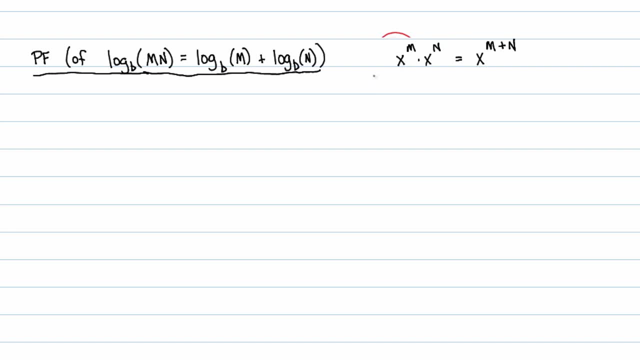 that it does stem from that property, because logarithms and exponentials are inverses of each other, so they should have some properties that are very, very similar. So now to the proof. And to prove something in mathematics you usually have to either start with some supposition. 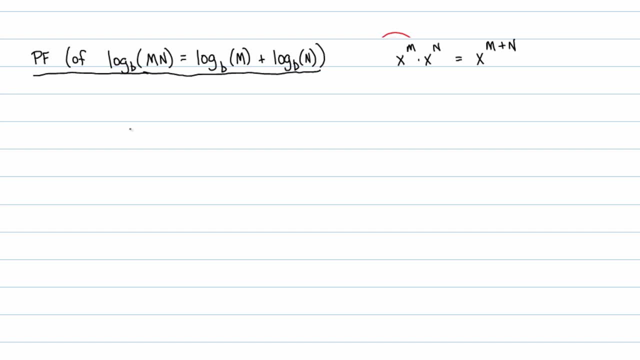 or something, or start with one part of your equation. in this case, I'm going to say: let's take a look at this stuff right here. I'm just going to try to, you know, figure something about, out about these two forms. I want to know what they're equal to. 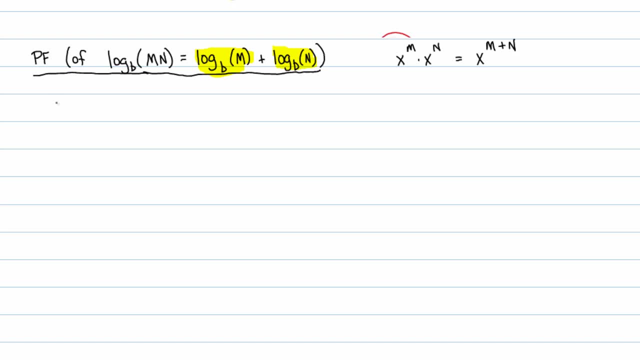 I don't know why. I just want to. let's just say so. let's go ahead and let log base b equal. well, I don't know what it equals to. well, if I don't know what it equals to, then I'll just call that x, because I have no idea what it really equals to, right. and since I did that, 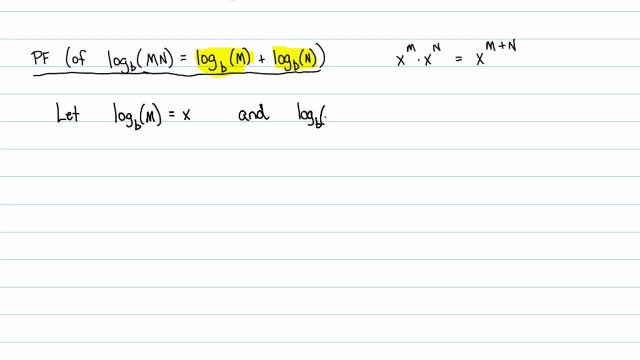 there. I'll just go ahead and say log base b of n is equal to good letters y. okay, so really what we're talking about is that log base b of m times n is just x plus y. that's, we're just Pretending for a moment. we don't know what those, those values are, and actually we don't. 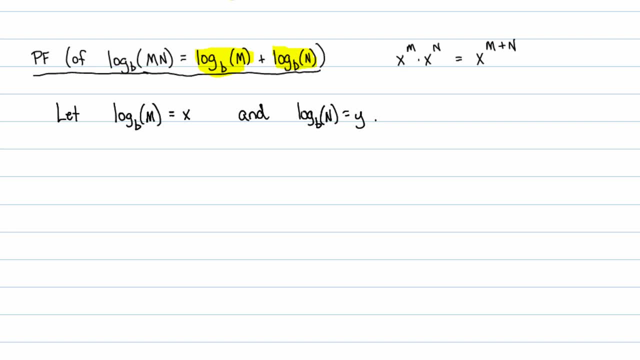 even know that log base b of m times m n is equal to this. we're just. we just want to find out if it's equal to that. So right now, all I know is I have log base b of m and log base b of n and I don't even 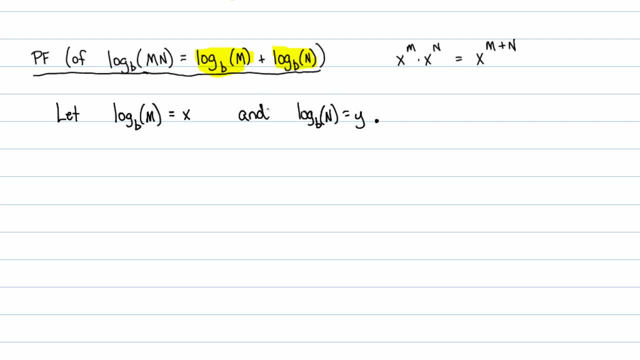 know what they equal, so I call them x and y. The only thing I could do with these is really transform them into exponential form. so using a circular argument here I could say: Well, this means, Or this implies- I guess It's a good way of saying that this implies- that b to the x, power is equal to m. 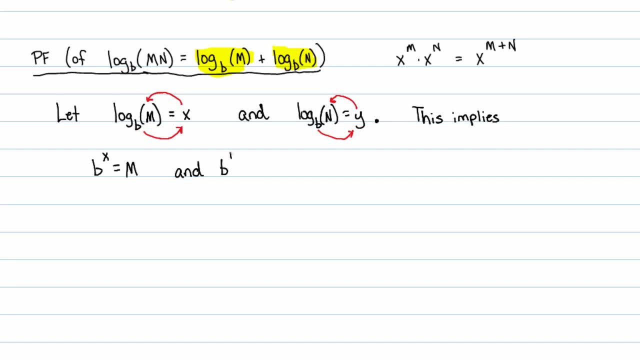 And well, b to the y, power Is equal to n. Well, this doesn't seem to be helping me. I don't. I don't think we're getting anywhere, so let's go ahead and focus in on instead 30.. 30., 40.. 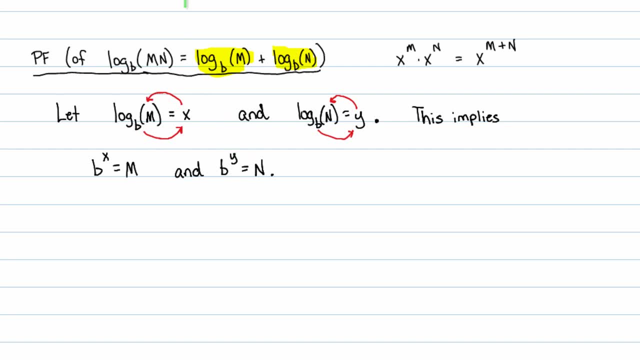 50. 50. 75. 76., 76.. this other part, because it doesn't seem. it seems like i'm going in circles here, so let's now zoom in on this bit right here. let's just see what this turns into. so i'm trying to show that this 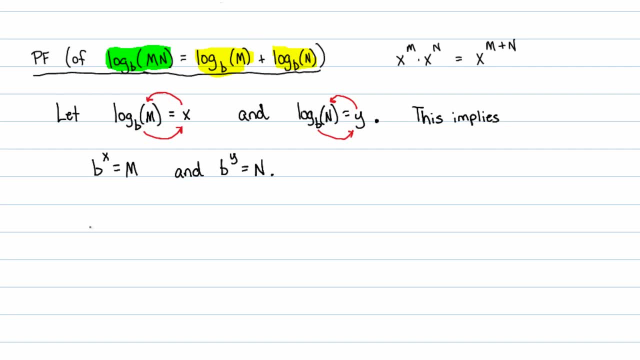 green part is equal to some of those two yellow parts there. let's see. so i have log base b of m n. by the way, i'll write thus: log base b of m n. well, hmm, i don't know what that equals to. but wait a second. i know that m is equal to b to the x and n is equal to b to y. i don't know what x and 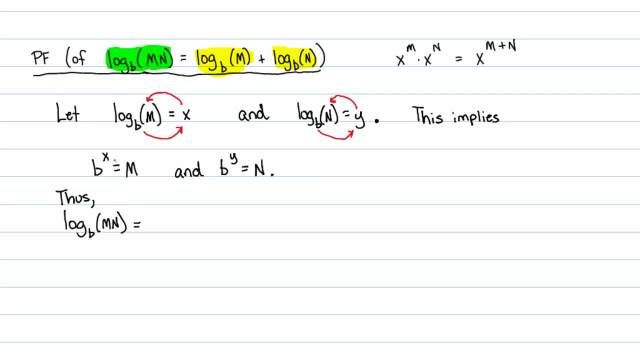 y are. but at least i know that m is equal to b to some power x and n is equal to b to some power y. so i'll just go ahead and write that in there log base b of instead of m. i'll replace that with b to. 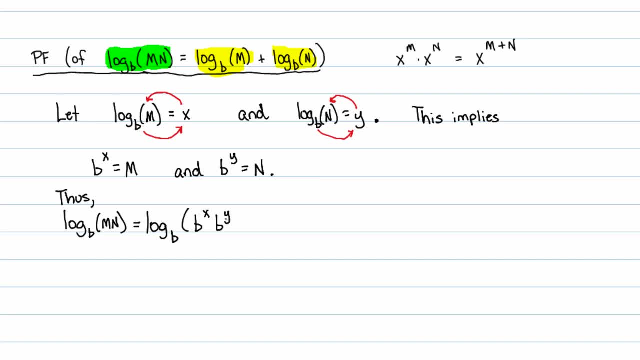 the x instead of n. i'll replace that with b to the y power. wait, i have a property actually that i could take advantage of here, a property of exponentials. so focus inside this parenthesis here: b to the x times b to the y. well, that's just. 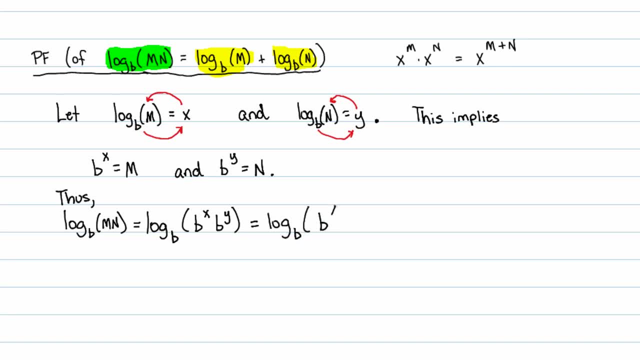 b to the x plus y. okay, well, i don't know what to do now. maybe i could resort back to looking at one of my properties here. see, uh, i have log base b of b to a power. let's see. oh look, look right here. log base b. 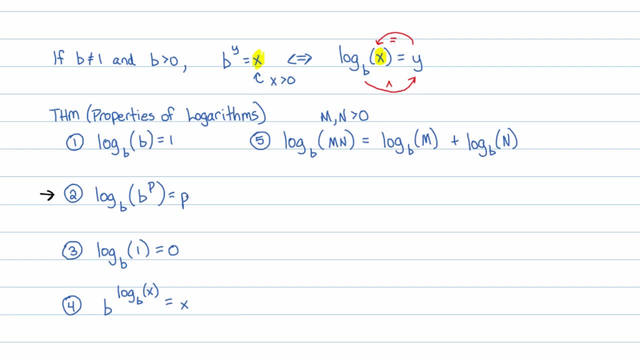 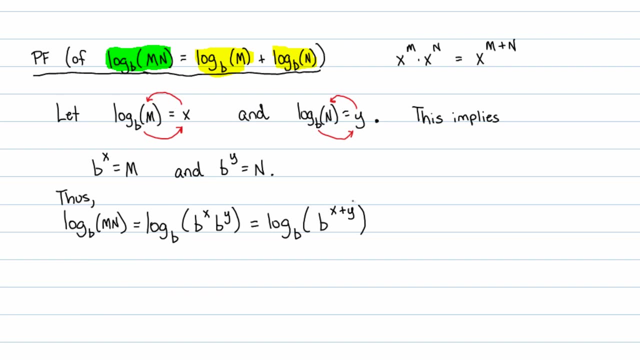 of b to a power is just the power. so log base b of b to this power, x plus y, is just should equal, just the power itself: x plus y. huh, that's pretty cool, okay, but wait a second. i don't want to end up with x's and y's, i want to end up with these logs and stuff like that. do we have? do we know what x? 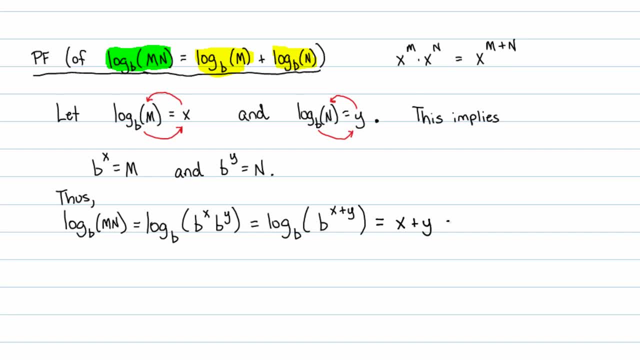 and y were originally sure we do. x is just equal to. from this statement right here that we started with, x is just log base b of m and y is just log base b of n. so i'll go ahead and fill those in. so x is just log base b of m. we have a plus sign and then y was just log. 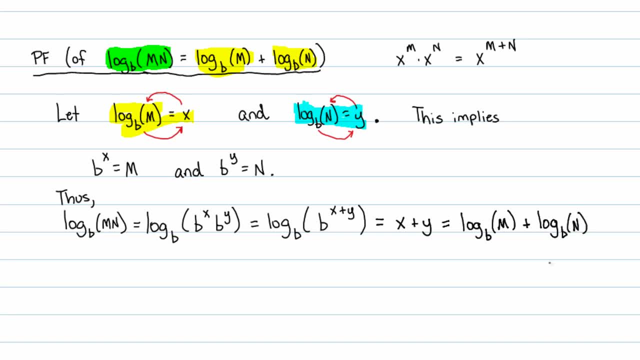 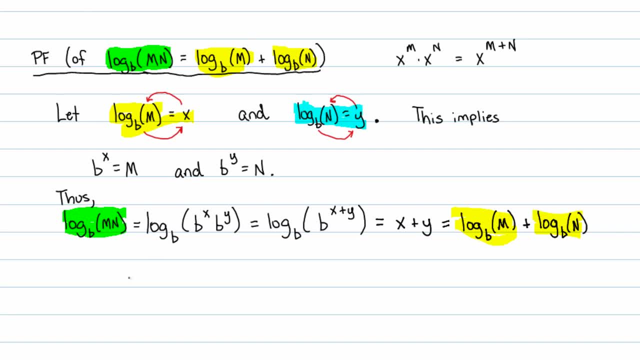 Again, I've just proven that log base B of M times N is equal to log base B of M plus log base B of N. Now that is pretty cool. QED means end of proof, quota rat demonstratum. so it has been proven. 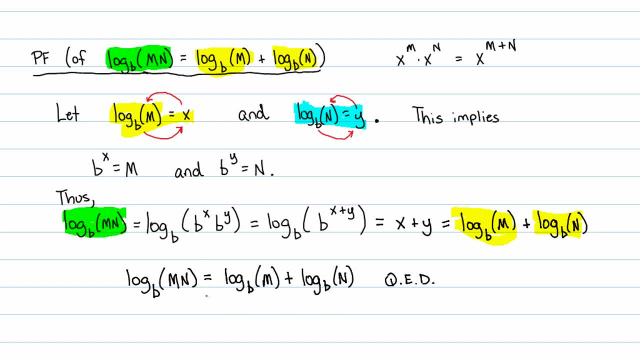 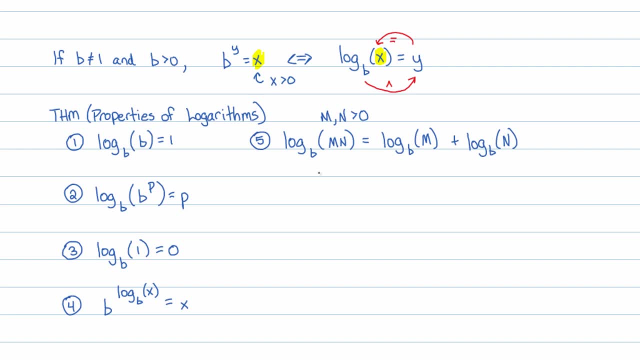 This theorem, This theorem, which is our fifth property here, is a very important theorem to use for any time, any time that you're working on a section in mathematics for properties of logarithms, but otherwise I rarely use this theorem, It's only really used in a proof. 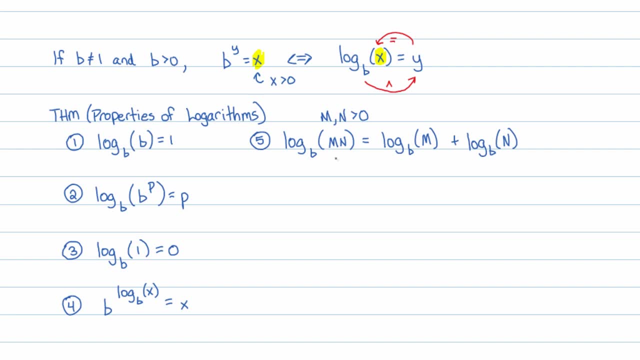 later on, in my opinion, and you use it obviously in this section. you know if you're doing homework in a section that requires properties of logarithms. but the most powerful, The most powerful theorem in logarithms we have not even yet stated, so we'll get there in a moment. 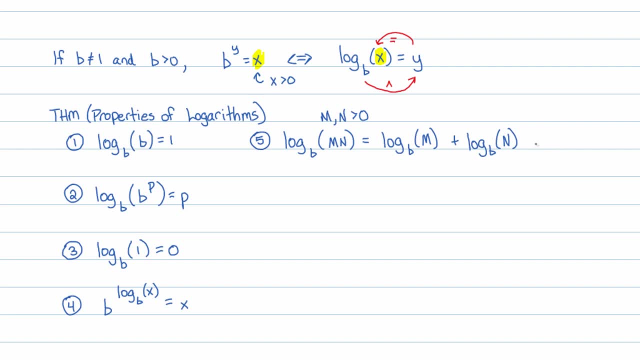 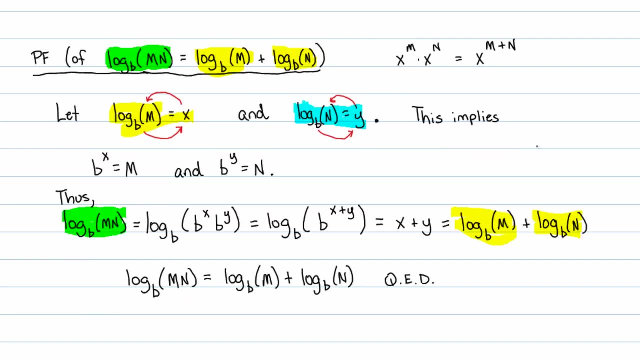 So this one, by the way, is one that I often tell students they have to kind of memorize, because it's not one that's easy to prove. You saw the proof here. It's a little convoluted, It takes a little thought. I would love it if you could wrap your mind around it. 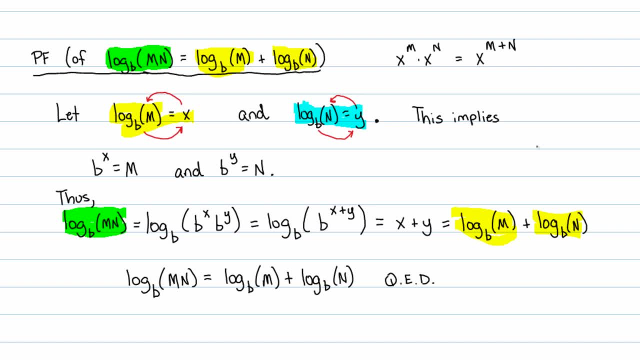 and I would. that'd be great if you could. You'd be an excellent student if you could. but it's very difficult to just prove it on the fly unless you have the proof memorized. So each of the other ones, like property 1,, 2, and 3, those pretty much fall out really quickly. 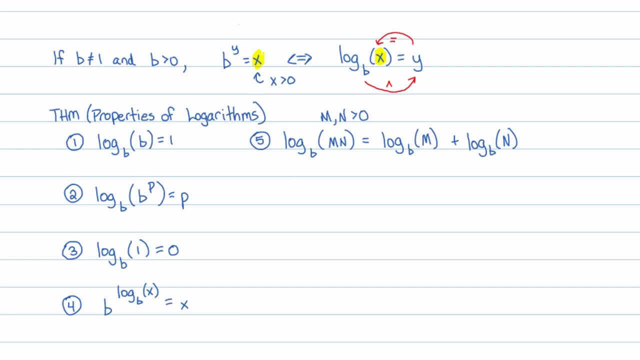 Even property 4 is okay, but property 5 is very difficult to prove if you forget. Same thing with property 6,, actually, but as long as you know property 5, property 6 should be okay. Property 6 is just saying that the log base b of m divided by n is equal to. 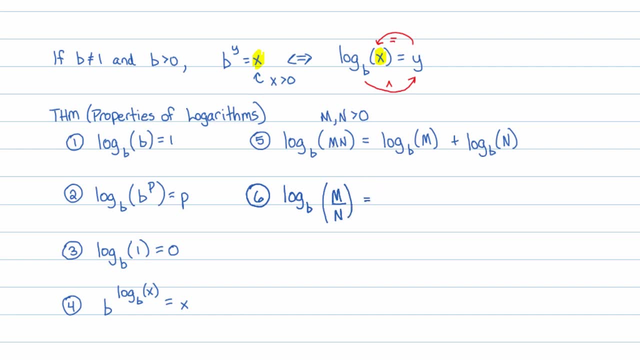 Well, if When we multiply, When we multiply, When we multiply m times n on the inside of the logarithm and that breaks out to an addition of logarithms, then a division should break out to a subtraction of logarithms. I mean that hopefully makes some sort of sense. 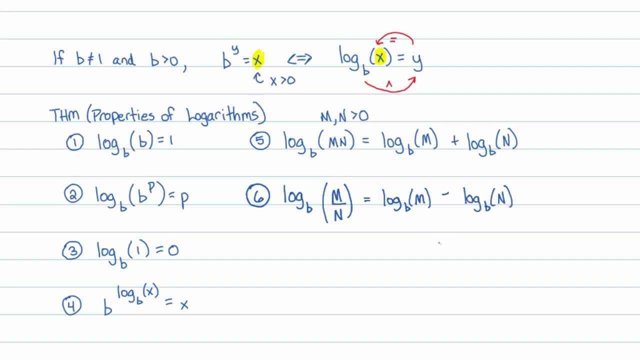 And I won't prove this. This is actually The proof of this- is almost exactly like the proof of the one we just did, but I will justify it. The justification, The justification is- Is more- Well, maybe not a justification, but more of a correlation with exponential functions. 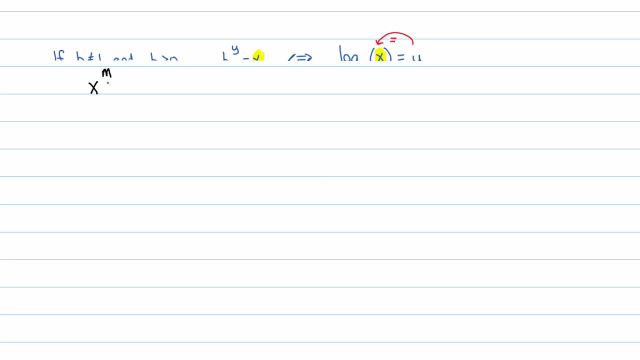 Again, recall that with exponential functions, if you have x to the m over x to the n, in other words you have a division. it leads to x to the m minus n And that division led to a subtraction. And the same thing is true with our properties here. 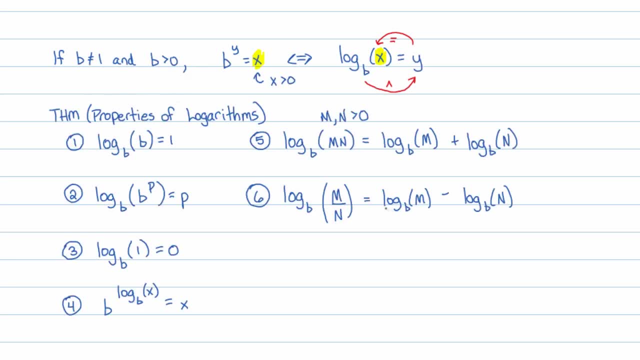 This division breaks out and leads to subtraction. Just remember that it's m times n on the inside of parentheses breaks apart to the sum of two logarithms, and m divided by n on the inside of parentheses breaks out to a subtraction or a difference of two logarithms. 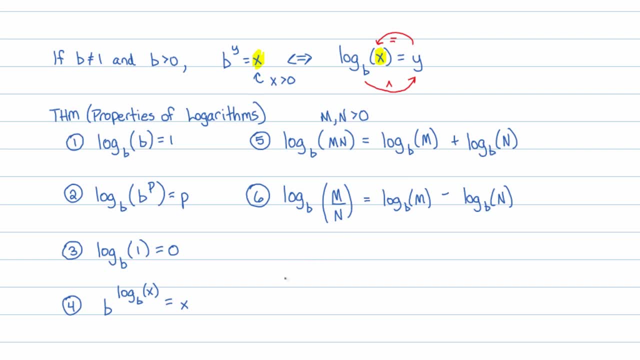 But those two are kind of inconsequential to me. The one that I really, really, really love, and probably the most important one that you'll- The most important theorem, I think, in my opinion in logarithmic functions is the seventh one. 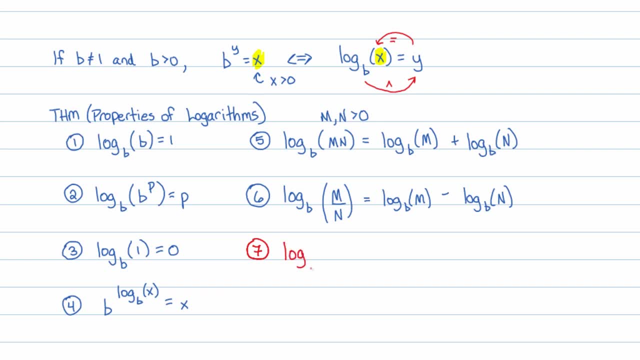 This is the basis for solutions of logarithmic equations. The log base b of any number to the p power is going to equal p times log base b of x. So log base b of x to the p power is just p times log base b of x to the p power. 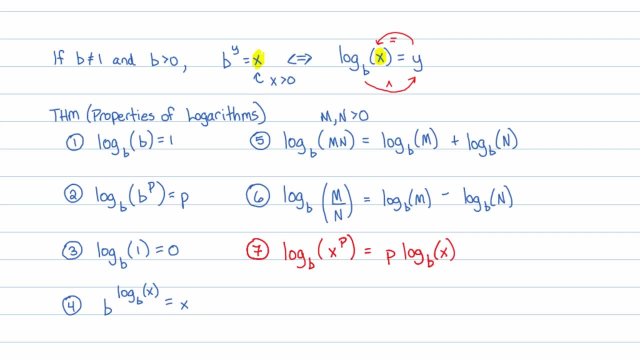 In other words, a lot of students love to see the action of pulling the exponent out front, And that's exactly what happened. We took the power of p and pulled it out front, And this is the one where I often say is really the backbone of all logarithms. 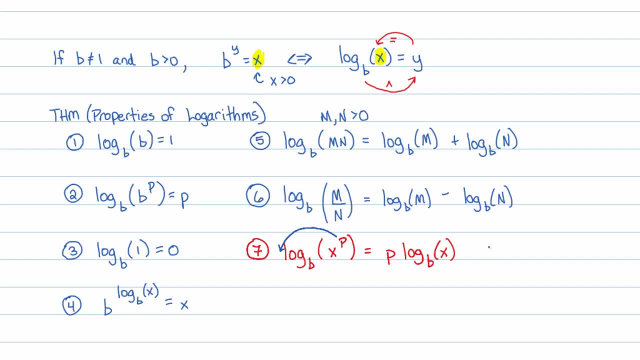 This is the one that allows us to really understand that logarithms undo exponents. In other words, if you take the logarithm of an exponential function, the power can pop right out front, So it unlocks exponents. This property extremely useful. 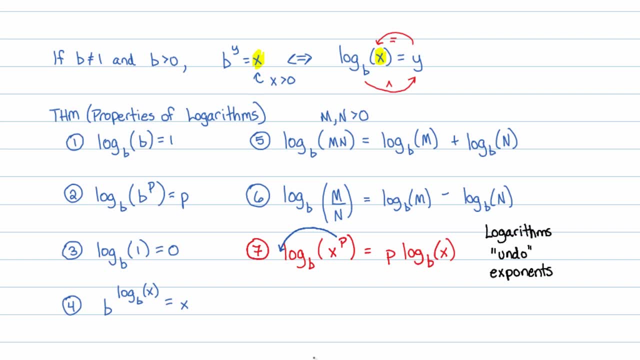 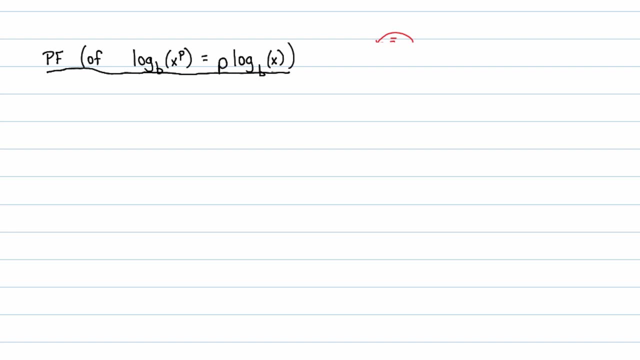 The proof of it is actually not so bad. The proof of the log base b of x to the p is equal to p. log base b of x goes something like this: You start with log base b of x to the p power, So that's log. 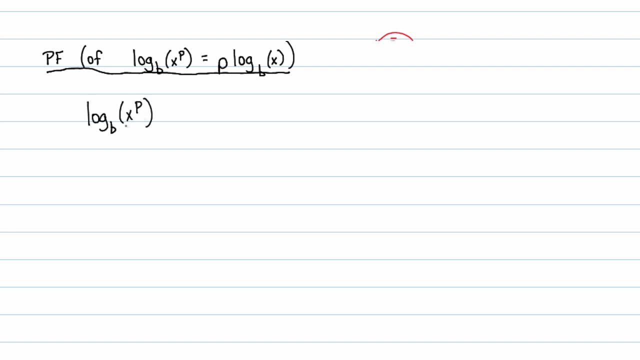 Base b of x to the p power And pretend as though nobody told you what it's equal to. The only thing that I could really do if somebody said I don't know what this is equal to, all I could do is say that's log base b of x. 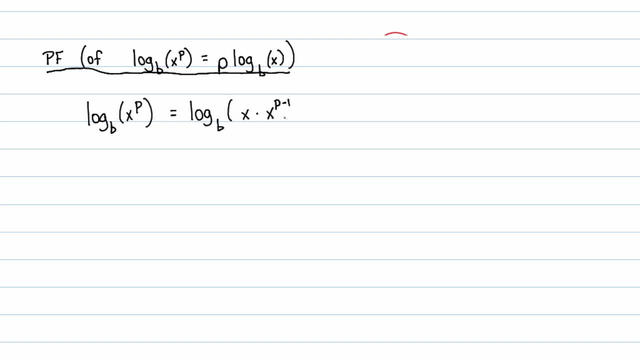 times x to the p minus 1.. Remember, x is like x to the first. So if you multiplied these two things- x to the first times x to the p minus 1, means you add their exponents right, So that'd be x to the 1 plus p minus 1.. 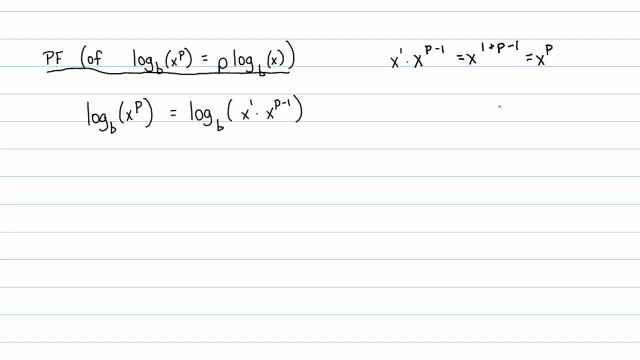 The 1s will cancel and you'll get x to the p. So all I'm doing is just taking out 1 power from that x to the p. So there we go. We have it right there, But wait a second, We have a theorem here. 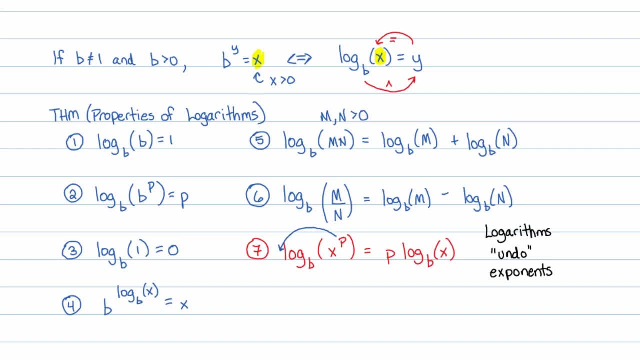 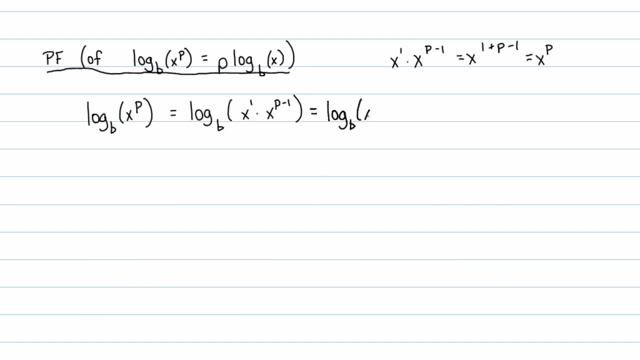 this number 5. that says if I have the product of two things inside a logarithm that I can break it apart into an addition. So that means I can break this apart into the log base b of x plus the log base b of x to the p minus 1.. 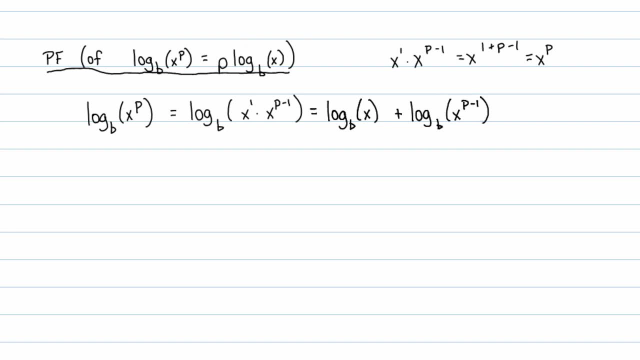 And then you think: well, that looks nothing like this. Well, it doesn't, But hold on a second. that's equal to log base b of x plus this log base b of x to the p minus 1, and then I'm going to break this apart. 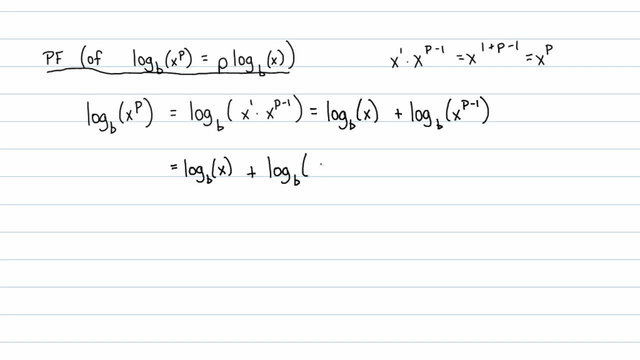 and I'm going to do the same trick again. That's log base b of x to the first times, x to the p minus 2 now. So I'm stealing another power away And again I can break this apart into an addition. 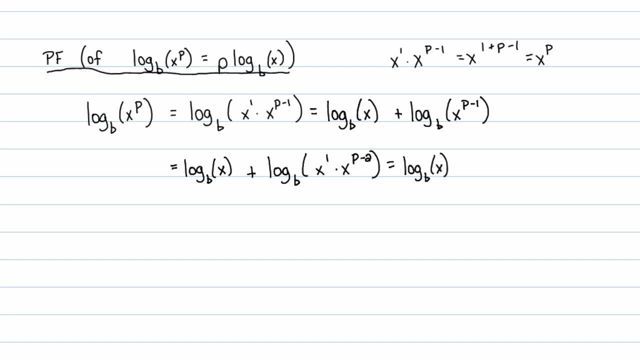 That's going to be log base b of x for this first little bit right here. That's just that Plus. now I'm going to break up this logarithm: Log base b of x plus log base b of x to the p minus 2 now. 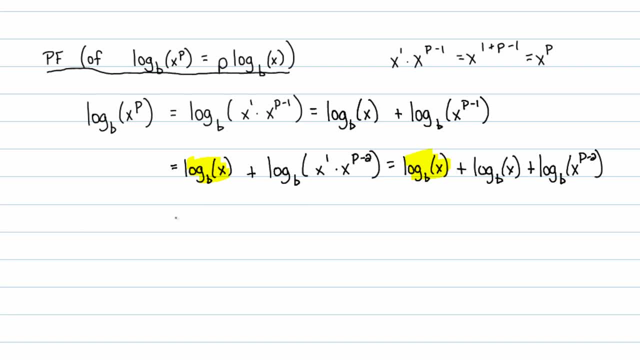 Wait a second. I have two of those log base b's of x's, so let me just write that down. I have two of those log base b of x's plus log base b of x to the p minus 2.. Well, I can continually peel off like this. 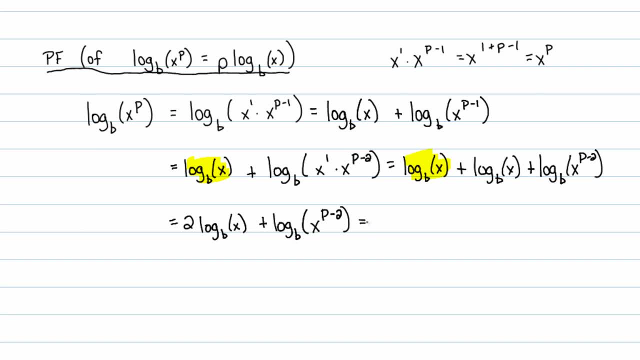 You can see like I could do this step again By just stealing another power out of this p minus 2, so it becomes a p minus 3 power, and splitting that again Where that two log base b of x is. just me rewriting this little bit right here. 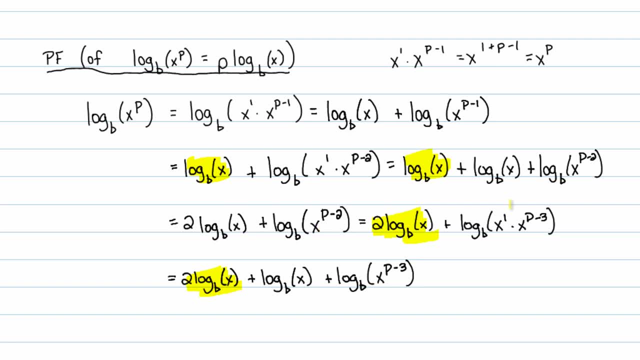 So these two match up. And then the last two terms- here are just me splitting this logarithm- And of course the first two terms there will combine and become three: log base b of x And then plus log base b of x to the p minus 3.. 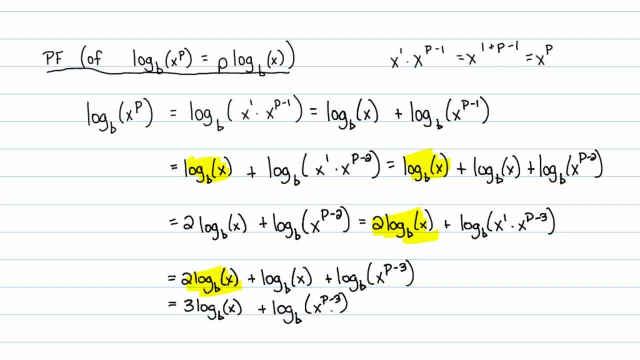 Well, okay, you can see this pattern is going to continue. We'll keep stealing powers away from this. So equals dot, dot dot. We'll keep stealing powers away from it until we've stolen all the powers from it. Well, if you steal all the power from it, you stole p of them. 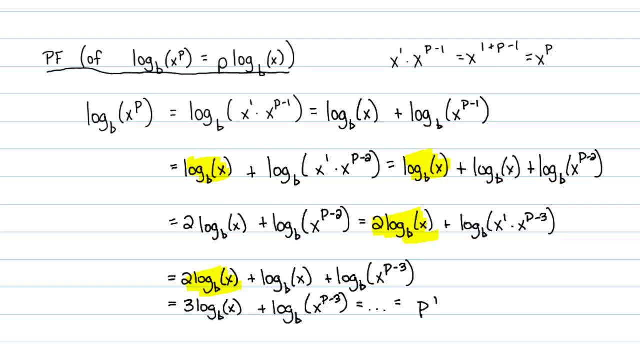 So you will have p of these log base b of x's. So that's it. So, through a chain of equalities, that's what we call this, a chain of equalities. log base b of x to the p is equal to this. 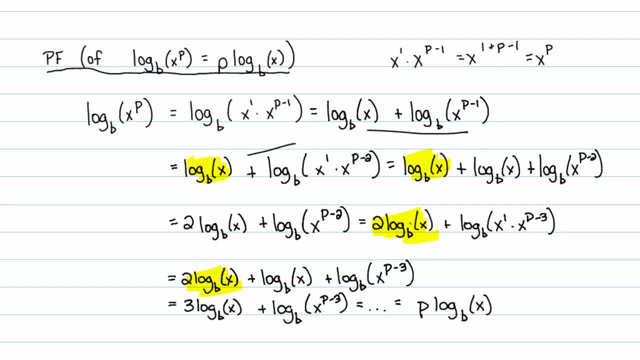 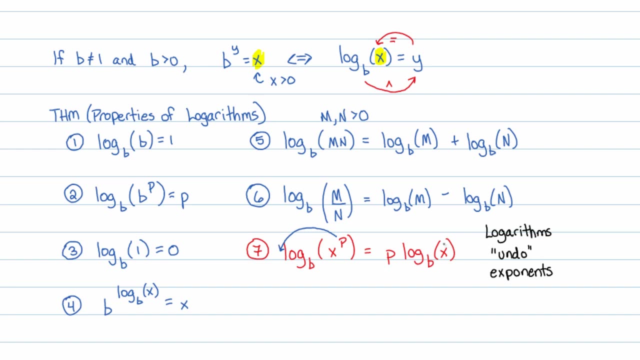 which is equal to this, which is equal to and equal to equal to, which all comes down to this. So, in other words, our theorem, log base b of x to the p must equal p log base b of x. Now, that's actually not the proof, to be honest with you. 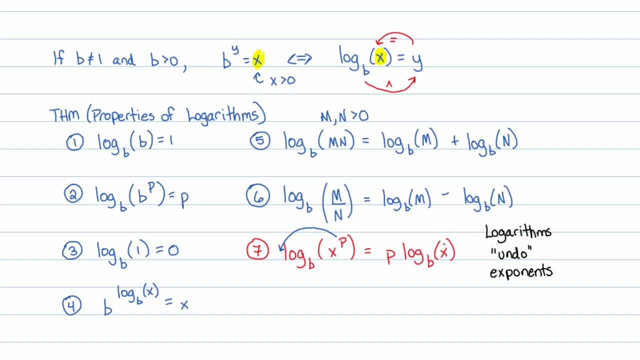 So if somebody wants to leave a message saying that's not the proof, that's just a justification, You're absolutely correct. A proof has to be done using more advanced techniques, but that's a great justification. If you're in precalculus, you can do the proof using induction. 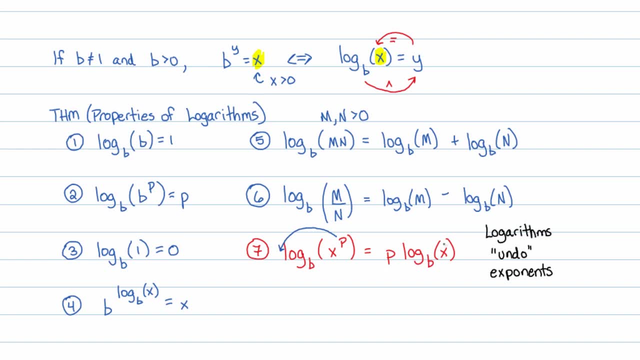 and that's how you would do the proof, or in calculus, whichever. Now there is, by the way, one other property which I rarely use, but it's an okay property. I'll write it in gray because it's a property that I kind of don't use that often. 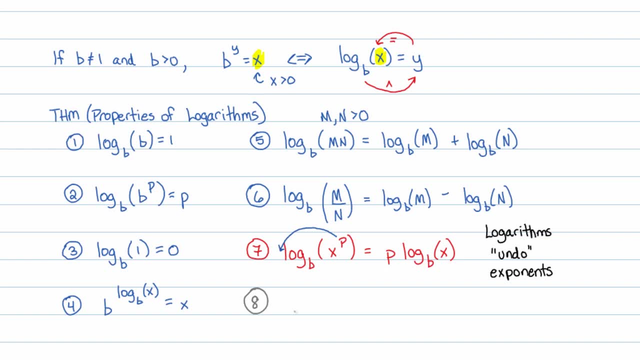 and anybody who's watched my lectures notices probably that I've only used it once. Turns out that the log base b of, let's just say x- let's just make our lives a little bit easier- can be rewritten as log base- anything I want. 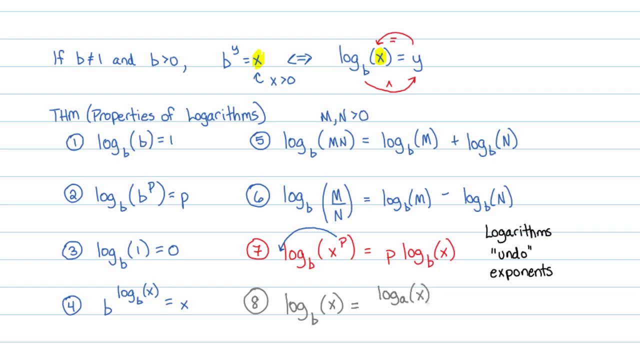 so let me say a of x over log base, a of b, As long as those a's are non-unit, in other words not one, and they're greater than zero, or they're positive. So they're positive, they're not one. 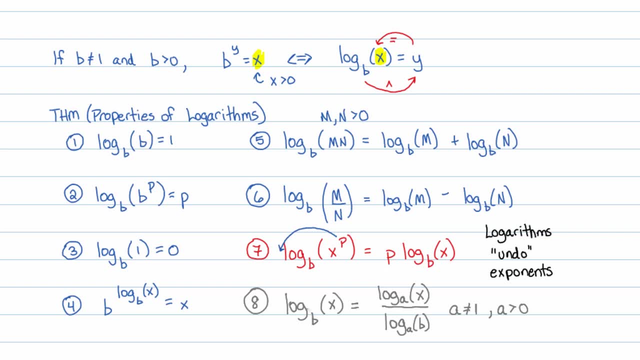 I could change the base of this logarithm to any number. I want Now notice the numerator and denominator both contain logarithms, right, And the base of each of those logarithms is exactly the same. So if you choose to change this to log base five, 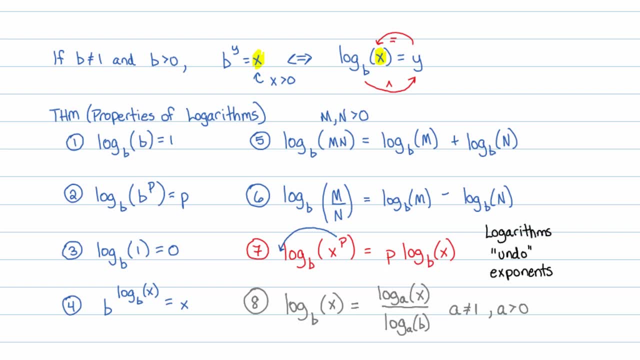 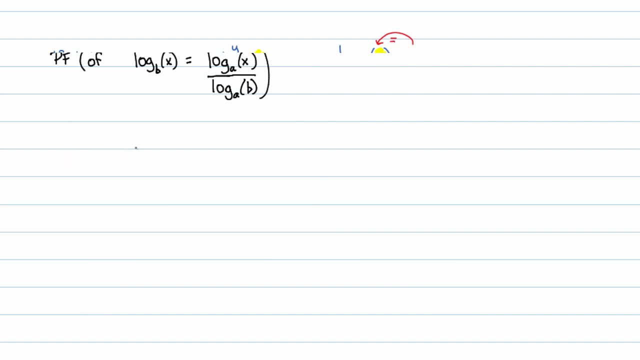 you better put a five for the logarithm base upstairs and downstairs. The proof of this is the proof of this property is actually not too horrible. All you need to do, really, is just take advantage of exponential form, And the proof also takes advantage of the last theorem that we created. 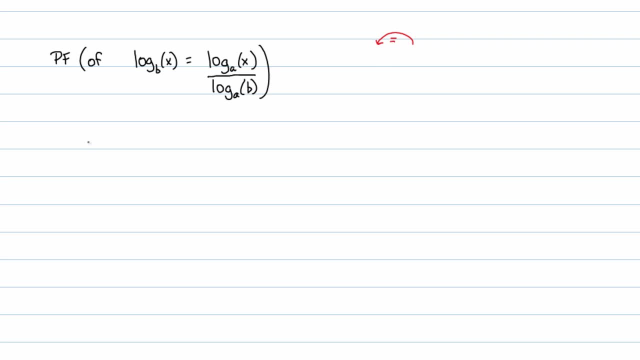 which is again the most powerful theorem in all of logarithms. So let's start by saying: let y equal log base b of x. Very simple start to all proofs is usually something very minor like: hey, I don't know what this is, so let's call it y. 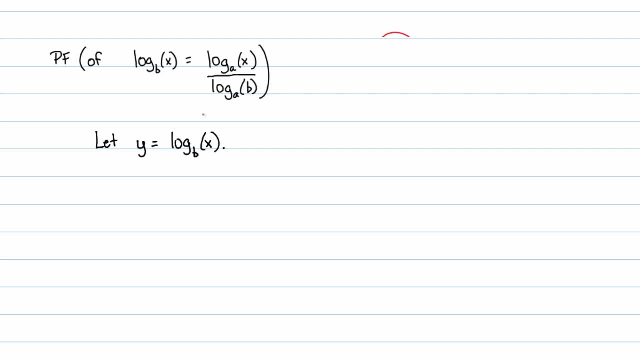 Now, if I'm starting with this and I can't just immediately say: well, therefore it equals log base a of x over log base a of b, because I haven't proven that yet, I have to somebody's throwing the gauntlet. Somebody said: prove this to me. 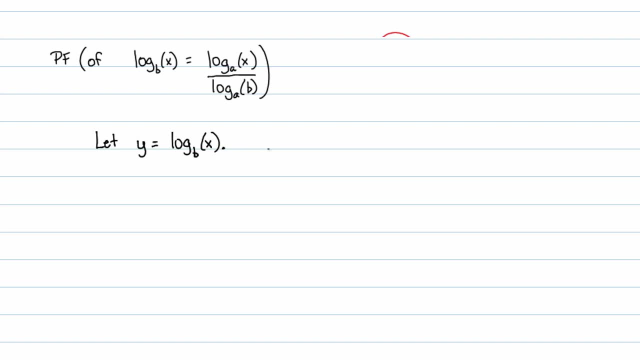 So I have to really take my time and prove it. One thing I know is that I could rewrite this in exponential form right: b to the y should equal the inside, Inside x. So in this case we'll say then b to the y must equal x. 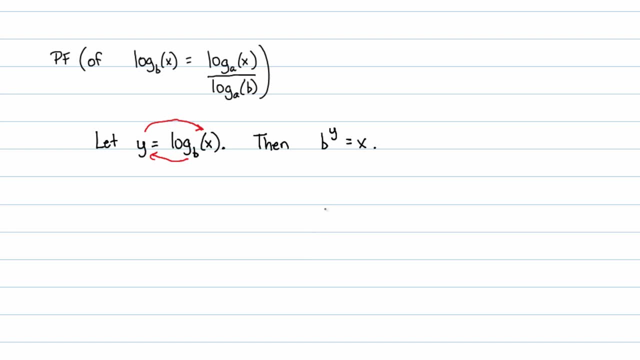 So you kind of stare at that for a while and we think and we're like: well, let's see, I want to get it to look like log base a of x over log base a of b. One thing I can do is, you know from equations, you can add 3 to both sides. 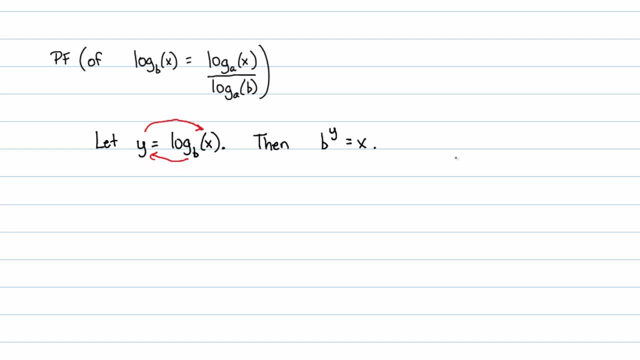 You can subtract 27 from both sides. You could divide both sides by pi. You could multiply both sides by 38.. You could take the square root of both sides. You could square both sides. You could also take the logarithm base, whatever you want- of both sides. 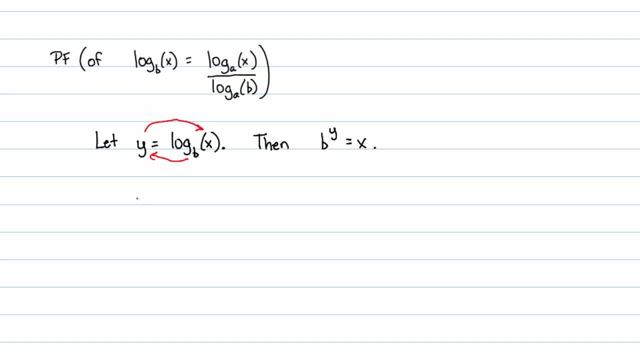 So let's go ahead and take the logarithm base a of both sides. I mean we could do that. It doesn't mean that it gives us an answer or anything, but let's go ahead and do that. So therefore, the logarithm base a of b is equal to log base a of x over log base a of b. 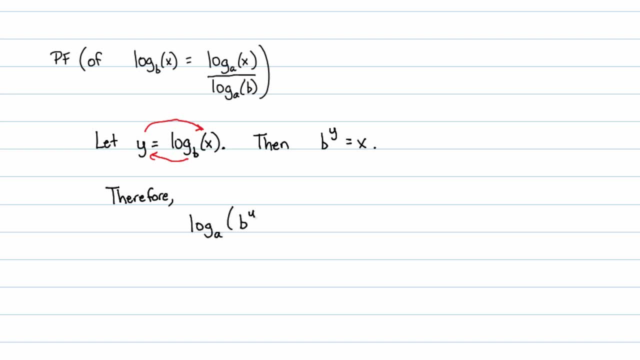 Base A of the left-hand side should equal the logarithm, again base A of the right-hand side. They have to be the same base, obviously, because I'm doing it at both sides. Whatever you do to one side, you have to do to the other side and it has to be the same. 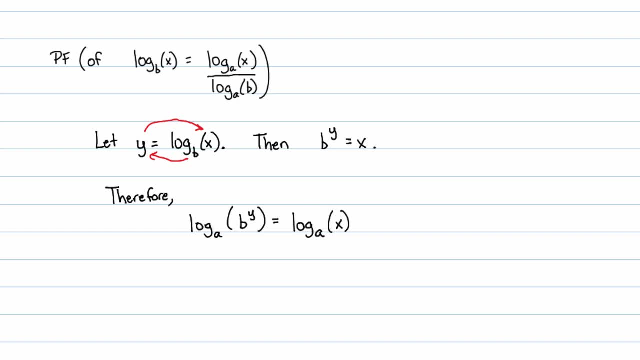 And now I can use that last theorem, which that last theorem said: log base whatever of whatever to a power. I could steal the power out front. Let me just show you the theorem, The theorem in red here Here: log base B of X to a power. 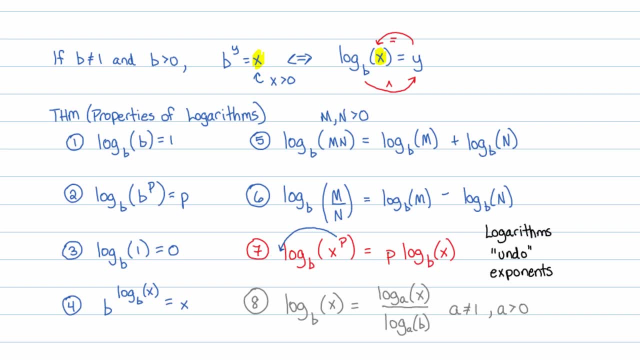 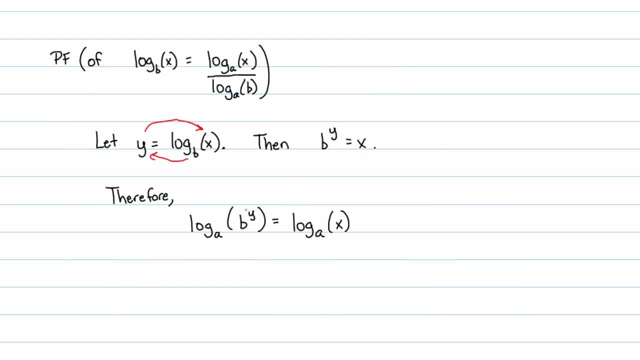 I could pull that power out front. Okay, So that's what I'm going to do in this proof. I have log base A of B to the Y. I'm going to grab that Y, the entire exponent, and pull that entire exponent out front here. 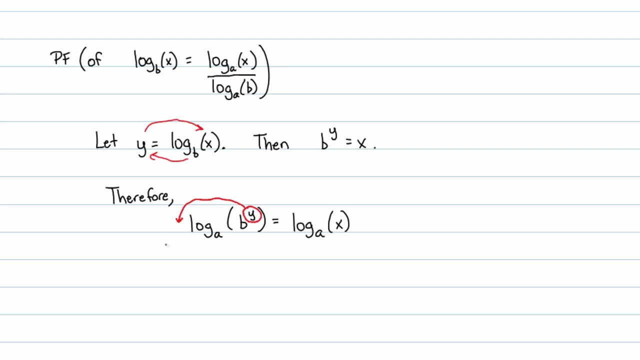 So I will get the following Y times: the log base A of B is equal to the log B, So I'm going to get log base A of X to the log base A of B. Now let's go ahead and solve for Y here. 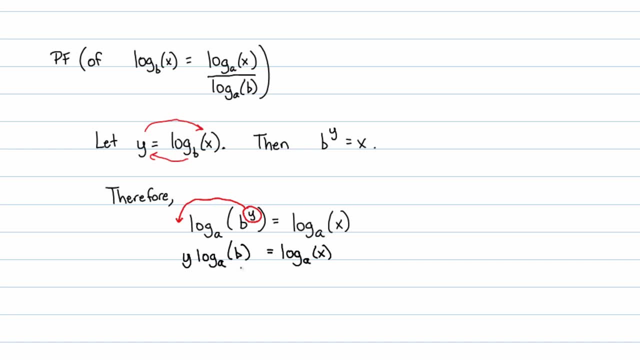 Because, well, it's an old habit. Plus, I see if I divide both sides by log base A of B, I'll get log base A of X over log base A of B, which is something in my final what I want to prove. 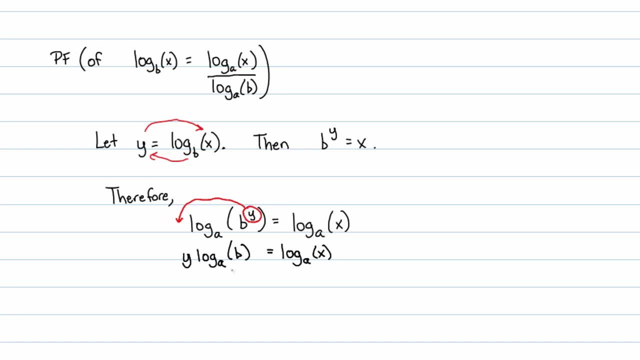 So let's see if that helps out. So I'll draw in blue here. I'm going to divide both sides by this picture. And remember, I like to talk in math, I like to talk about pictures. The pictures have to be exactly the same to cancel. 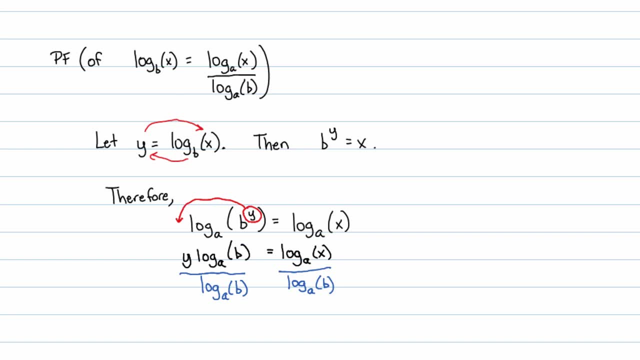 These two pictures are exactly the same, so they cancel out very nicely, And I'll get the following: That Y is equal to log base A of X over log base A of B. Now notice, I'm not canceling the words log base A. 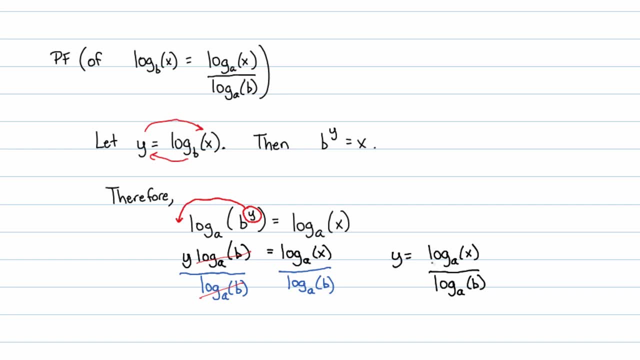 I can't do that Because this entire picture upstairs is not exactly the same as this entire picture downstairs. They cannot cancel, So you can't just cancel letters like that. These are functions. So they have to do something to X. Top one has to do something to X. 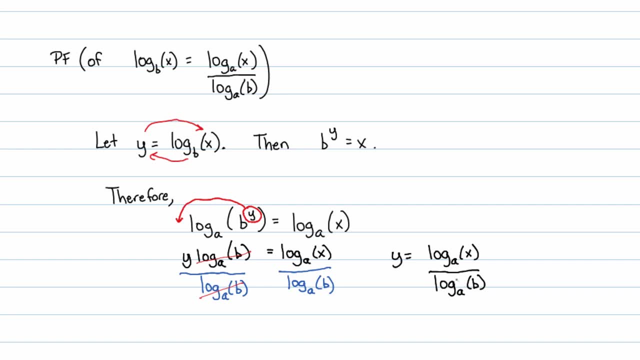 And the bottom one has to do something to B, And then, once it does that, then you might be able to cancel things, but not until you let that machine run. Well, this is where I want to end up, but it sure doesn't look like what I want to prove, right. 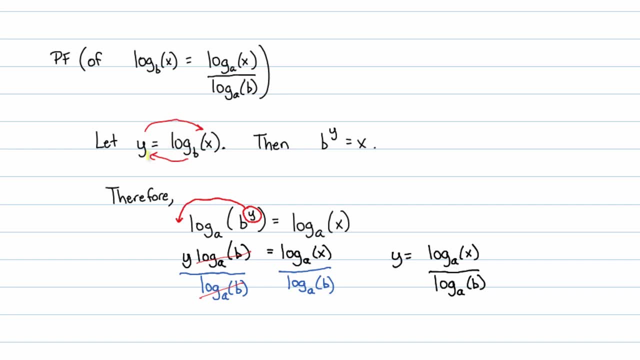 Oh wait, wait, wait, Hold on. Y happens to be equal to log base B of X. That's what we started with. Y is equal to log base B of X, So this Y right here is log base B of X. 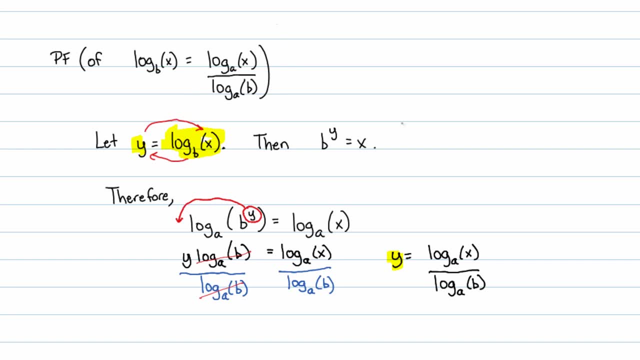 Aha, That means that log base B of X- this little business right here which is Y- is equal to this stuff: Log base A, Log base A of X over log base A of B. And there you have it. That's the proof of it. 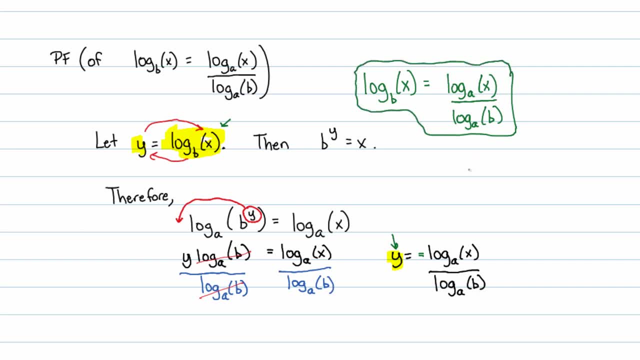 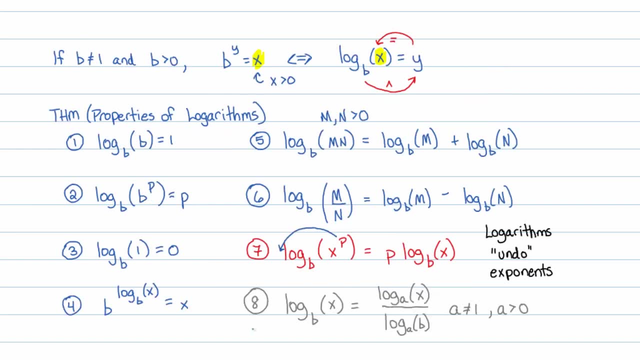 Okay, That's called the change of base formula. That's a proper name for it, I suppose. I suppose that's what everybody calls it in textbooks, But again, I generally don't use it because when I take the logarithm of both sides of a function, 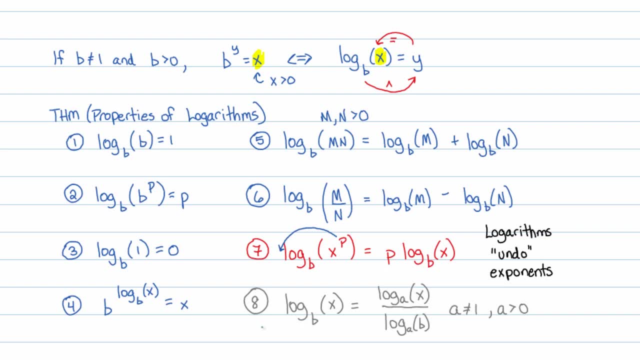 I generally take either log base 10 or log. I usually take log base E, which is something I haven't talked about yet, but usually log base 10.. Mainly because log base 10 is a logarithm that my calculator can handle. 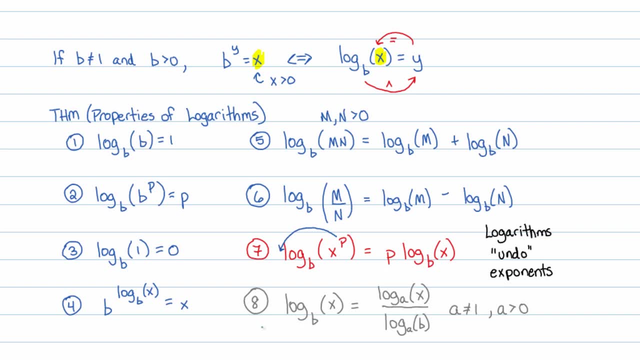 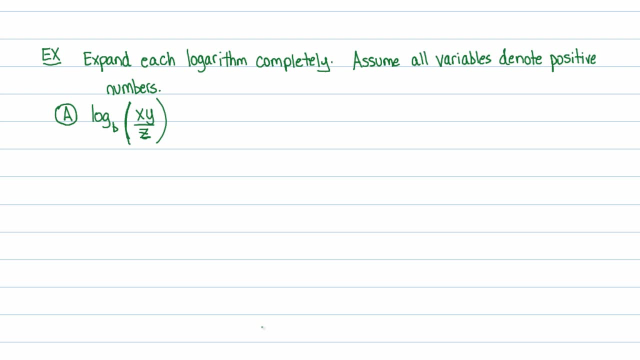 Why would I want to take log base 5 of both sides or something like that? That's ridiculous. So let's start going into the examples. Now that we have all the theorems down, let's start using them. So there are two basic styles of examples. 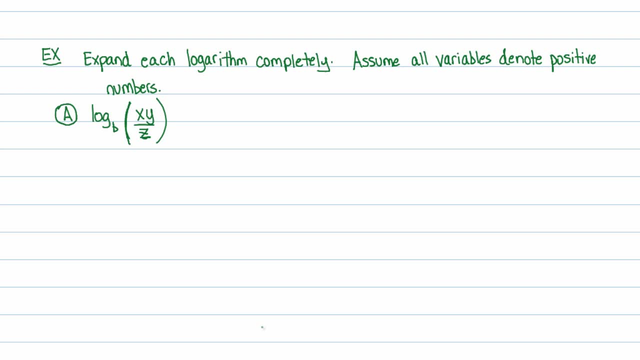 They're kind of, you know, just as typical silly textbook examples of expand And condense or contract. We're going to expand these logarithms completely. What that basically means is that you want to rip them apart to where they're just log. base B of X. 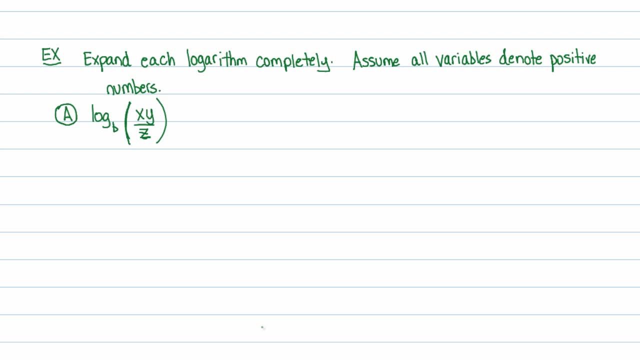 log base B of Y, log base B of Z. So you want to use properties of logarithms to pull this apart to its basic components. And the other little note here is: assume all variables denote positive numbers. And the reason why is because well, inside a logarithm, 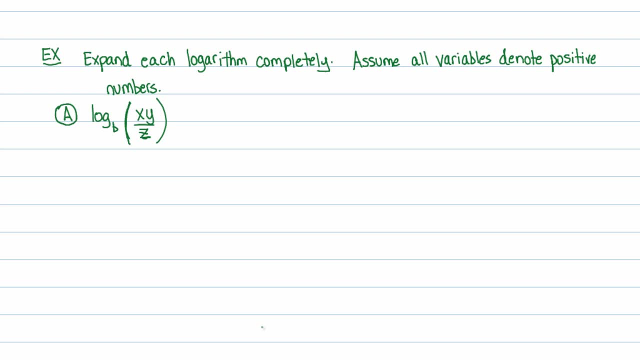 you must have only a positive number, okay. So that's what we would call the argument of a logarithm must be positive. So, using the property of logarithms here, let's see what we could do. Well, I see. first thing, you should follow the order of operations. 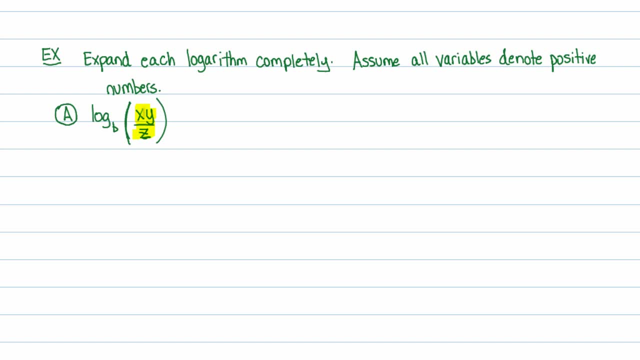 So you kind of focus in on the inside of the logarithm here And you see if you could simplify that first. Nothing really simplifies, so I can't really do anything. So I hop outside of the logarithm And I see if there's any work I can do. 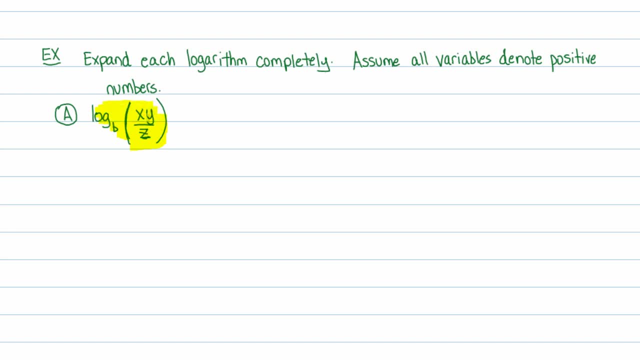 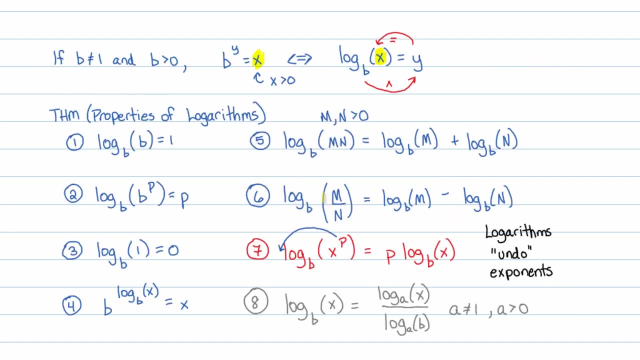 And I see, okay, I've got a logarithm with a fraction on the inside And I have a property. Let's see it's the sixth property here. If I have a fraction, I can write it as log base B of the numerator minus log base B of the denominator. 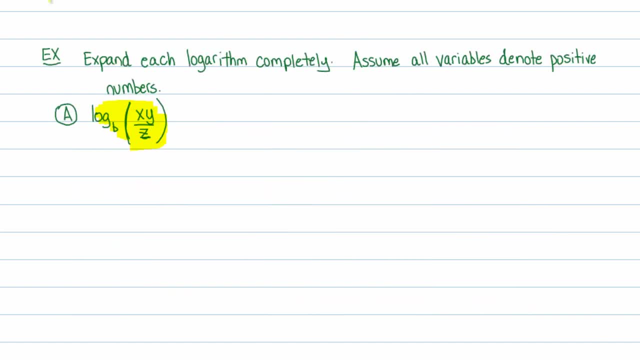 So I'll go ahead and do that here. I'll write this as log base B of that numerator, which is XY Minus log base B of the denominator, which is just simple little Z. Now, if you look through both of these logarithms, you have to ask yourself: are we done? 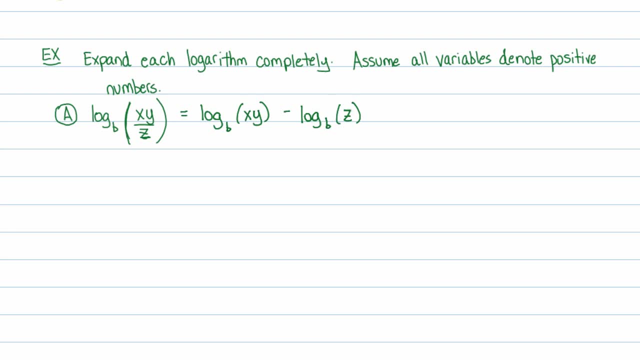 This last term is: you can't really simplify log base B of Z any further. It's just log base B of Z. There's nothing else you can say But this first logarithm. you see, I have log base B of a product. 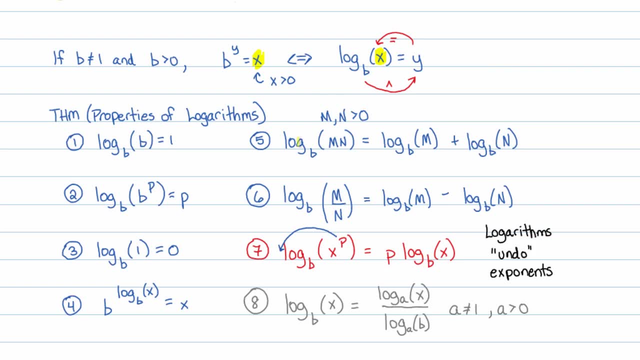 And I know I have a theorem That says if I have log base B of the product of two objects, it's going to be log base B of the first plus log base B of the second. So we get to split that apart. 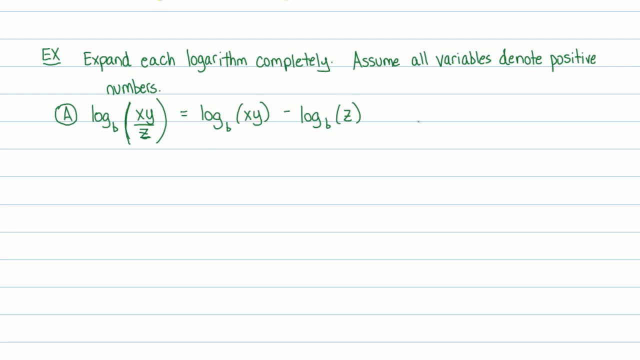 So let's go ahead and do that. It'll equal log base B of the first plus log base B of the second. And don't forget, you're losing log base B of Z on the end. Often I find that students forget They rewrite the last little bit. 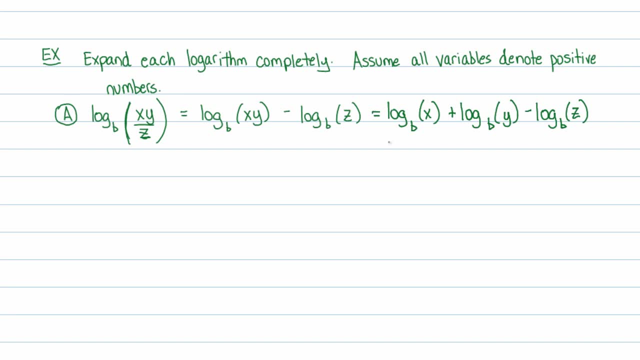 This is a fully expanded logarithmic expression Because, as you look through this, all the inputs to your logarithms are variables to the first power. That's the most important part. They just have to be single little variables to the first power. That's it. 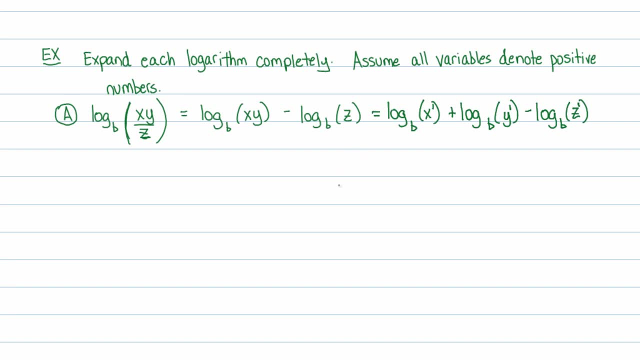 That's when a logarithm is completely expanded. So let's try another one here, The log base B of the fifth root of X cubed. Often root notation or radical notation and logarithms do not work well together, So you want to rewrite that in terms of rational exponents. 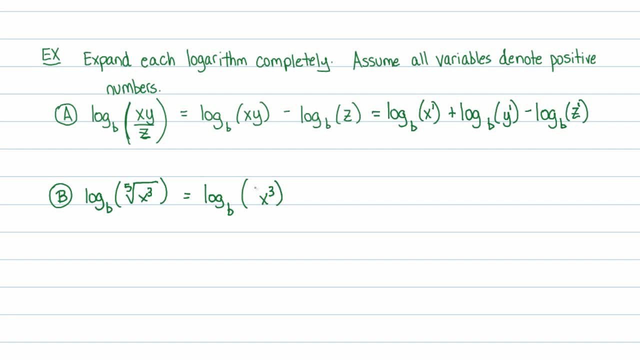 That's going to be X cubed being raised to the one-fifth power, Or in other words, it's going to be X to the three-fifths. Now this is not actually simplified yet. This is not expanded completely. We can use that property that says: oh, if I have a single variable raised to a power? 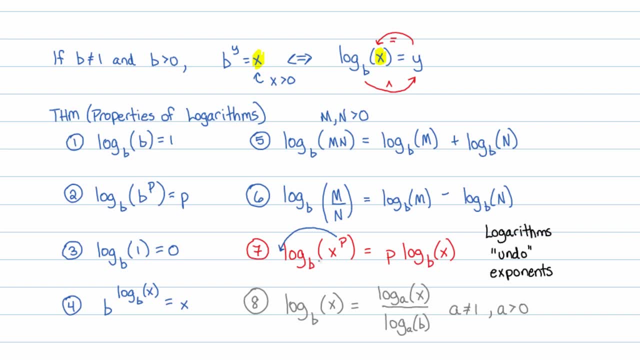 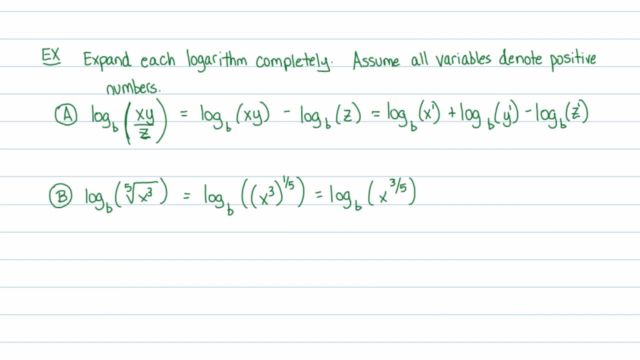 Do this one right here. If I have log base B of X to a power, I can pull that power out front. So here I have log base B of X to a power, I can pull that power, that entire power, out front. 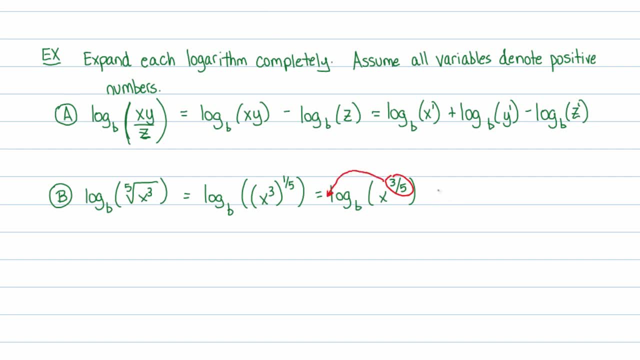 So here we go, Let's go ahead and do that. That'll be three-fifths, log base B of X. Notice now my logarithm has a single power on the X. That means we're done. So let's ramp it up a little bit here. 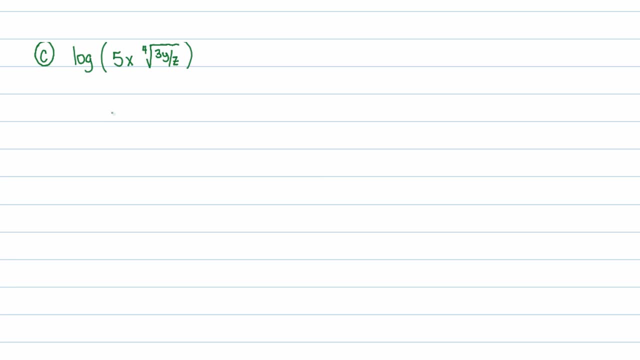 We have log of 5X times the fourth root of 3Y over Z. There's a lot of action going on in this one, So let's take our time. Let's see. I have a couple things being multiplied here, Actually three things being multiplied on the inside of this logarithm. 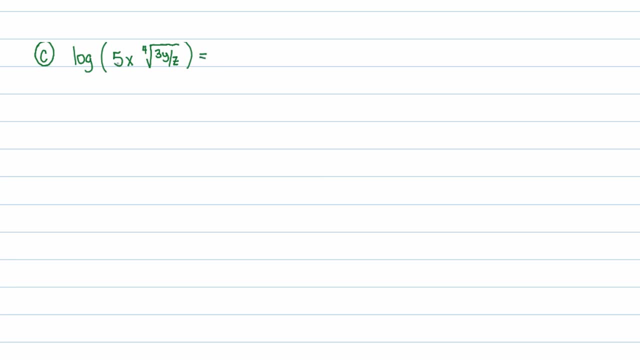 And so I'll have remember. when objects multiply, it leads to addition. So this is going to be log of 5.. Remember the base is 10.. I'm not going to write base 10 because there's no point. 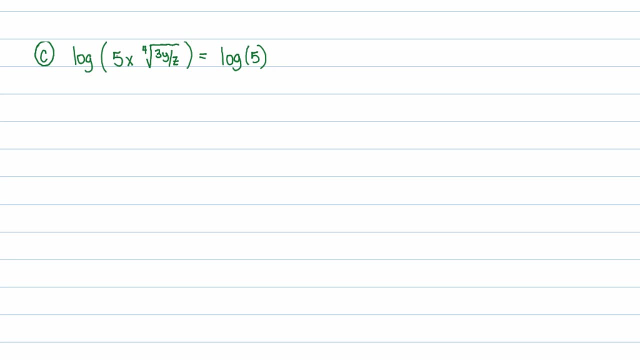 But it is assumed to be base 10.. So it's going to be log of the first factor plus log of the second factor Plus log of the third factor, which is the fourth root of 3Y over Z. Now those first two are actually pretty much nice and clean. 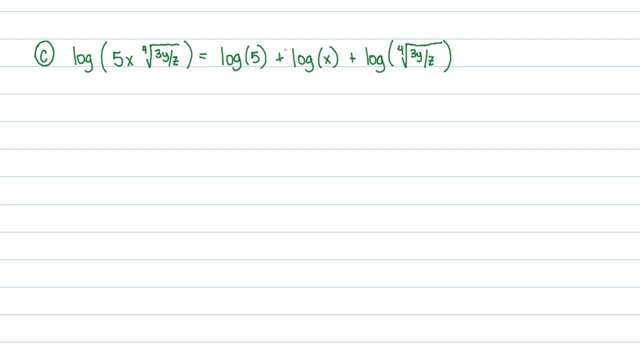 And, by the way, I don't know, 10 to the power. some odd power is equal to 5.. I have no idea what power of 10 turns into 5.. So that is a perfect form right there. You don't need to clean that up. 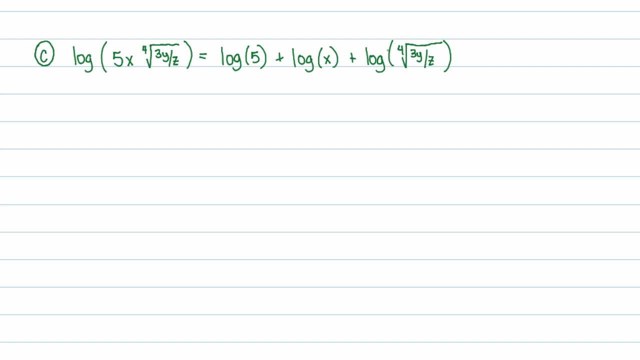 That's just log of 5, right there. But this last term, remember? I just told you radicals usually don't work well with logarithms, So I'm going to change that to rational exponent notation. So let's see, This is equal to log of 5 plus log of X plus log of, and I have a 3Y over Z being raised. 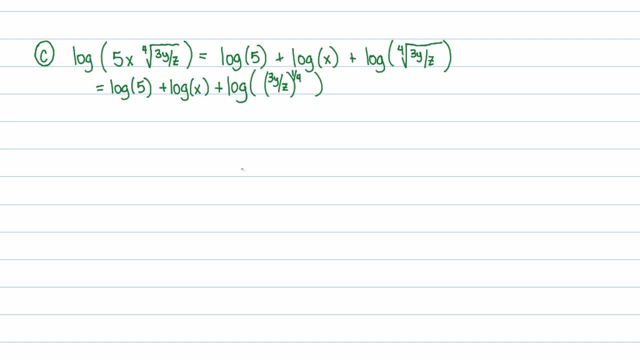 So I have a 3Y over Z raised to the 1 fourth power. Now I have a log of something raised to the 1 fourth power. It means that I could take that power and pull it out front. Remember that property. 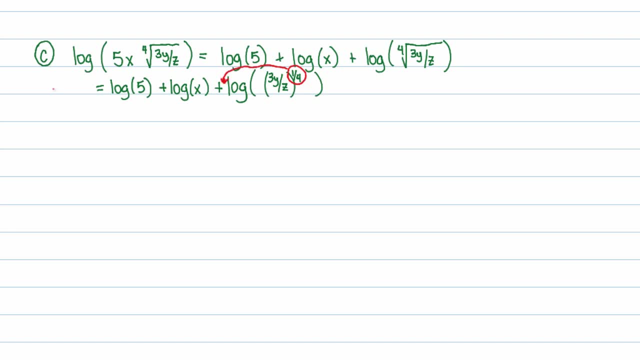 So you pull it out to the front of that logarithm, Not to the front of all the logarithms, but just that logarithm. So, rewriting: I've got to leave a little space here, actually, because it's a little cleaner that way. 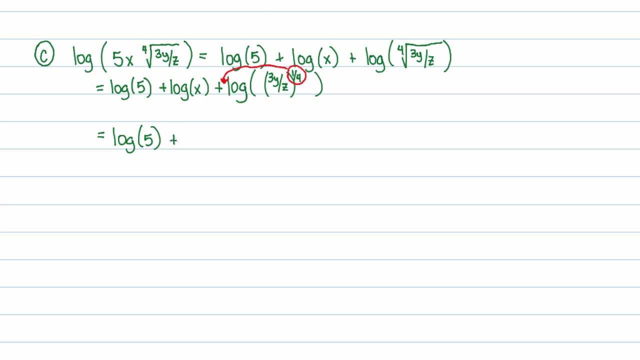 Log of 5 plus log of X Plus 1. fourth log of 3Y over Z. And now I see this 3Y over Z in here needs to be split apart. right, We'll have this numerator minus that denominator, or in other words a subtraction. 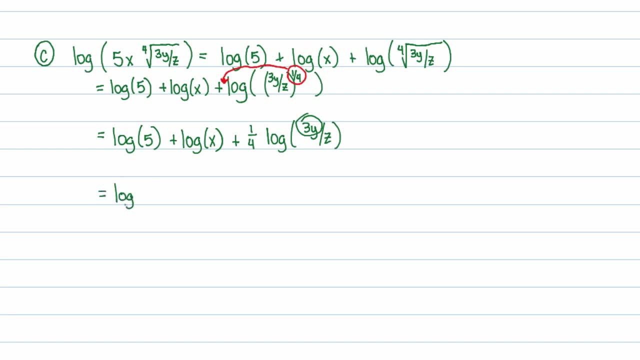 And here's where I want you to be very careful: Watch how I'm continually rewriting those first two terms. I'm making sure that I don't lose them. I also write that 1 fourth, And remember that 1 fourth is multiplying this entire log, right. 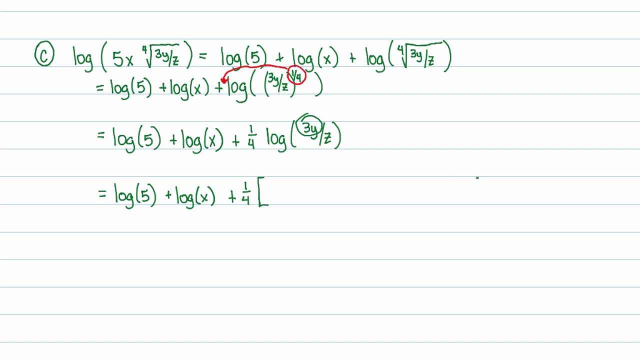 So when you rewrite this you have to write a parenthesis. This logarithm is going to break into the log of 3Y minus log of Z, But each of those objects is being multiplied by 1 fourth. So because that 1 fourth is multiplying this entire logarithm, 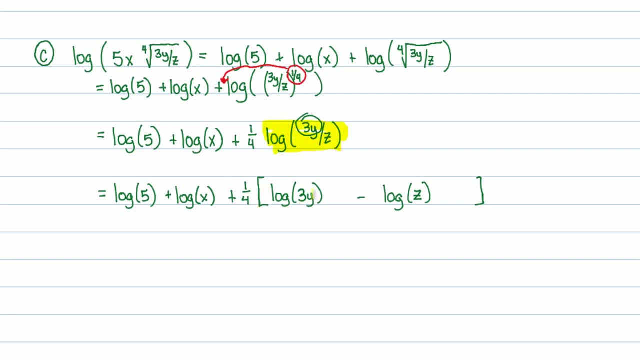 So I have to make sure I have to make sure that in the end, when I split it, it's still both of those are still being multiplied by 1 fourth. So this is the best way to do it: Just write a parenthesis on there. 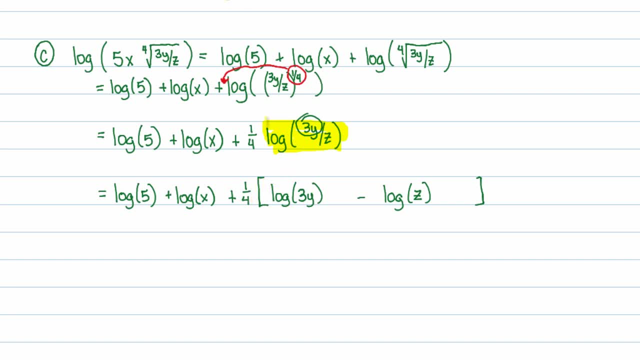 And you can leave the parenthesis there if you want, for a little bit, until you're done expanding. So let's go ahead and continue forward. That 3Y can even be split apart, right? So that's going to equal log of 5 plus log of X plus 1. fourth, 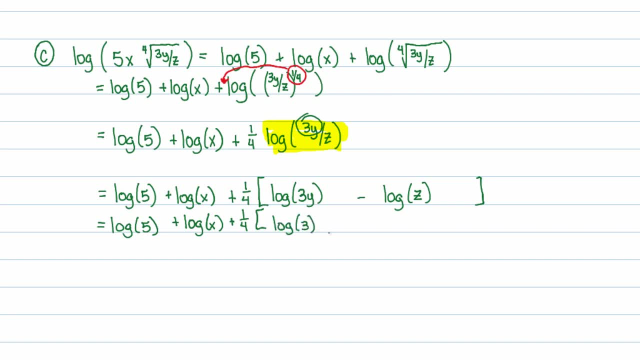 Times. log of 3Y 3 plus. log of Y minus. log of Z. End that bracket And, if you felt like it, you could distribute the 1 fourth through. A lot of people tend to like that, So we'll go ahead and do that. 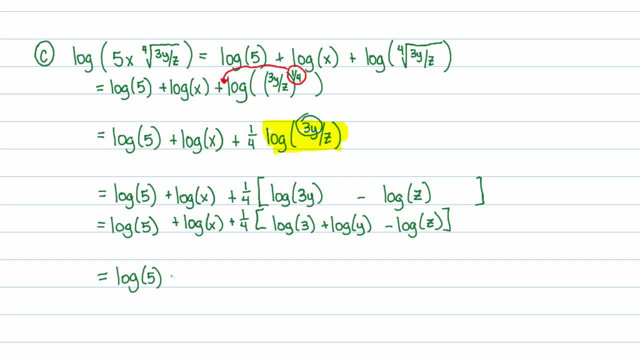 Log of 5 plus log of X, plus 1 fourth log of 3.. Plus 1 fourth log of Y, minus 1 fourth log of Z. Notice how I'm distributing that 1 fourth to each of those terms. You would like to see if any of these terms combine, but there are no like terms here. 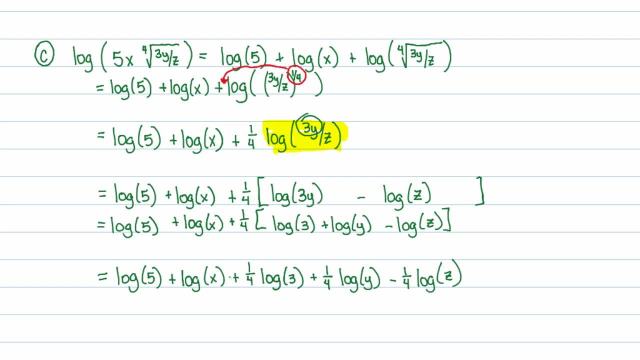 This is a log of 5,, which is not the same picture as this picture log of X, which is not the same picture as this picture log of 3, and so on and so forth. None of those are the same. 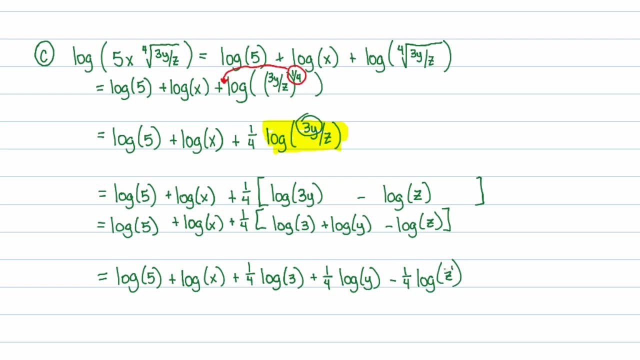 But these are all simple logarithms. They all have a number or a variable to a power- 1 on the inside. So these are all completely fine. That is completely expanded. Now, something I want to draw your attention to: to kind of start noticing shortcuts as you start working through these problems. 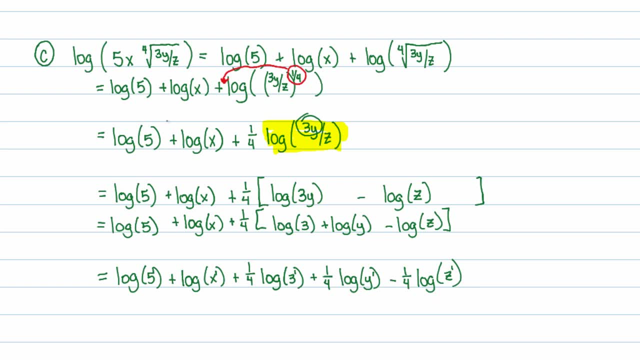 Notice that everything that was in a numerator, like for example, this 5 is 5 over 1.. This X is X over 1.. That 3 and that Y. Notice all of those items when in the expansion, I'll highlight them here. 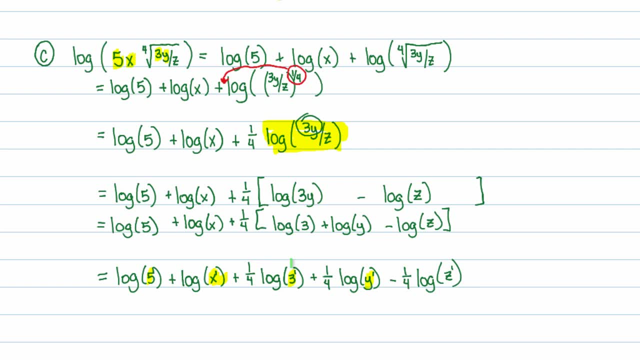 Notice that they were all positive And there is a plus on that log of 5.. Notice they're all positive And also notice that everything that happened in the that was originally in a denominator, which is that Z is negative. That is not a coincidence. 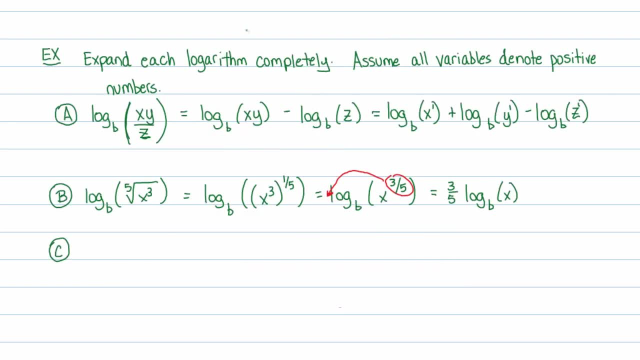 Go back to our first example. Notice we have XY in the numerator here And notice that when we got to our final answer, the logarithm with Y in it was positive and the logarithm with X in it was positive. Notice in our example that Z was in the denominator. 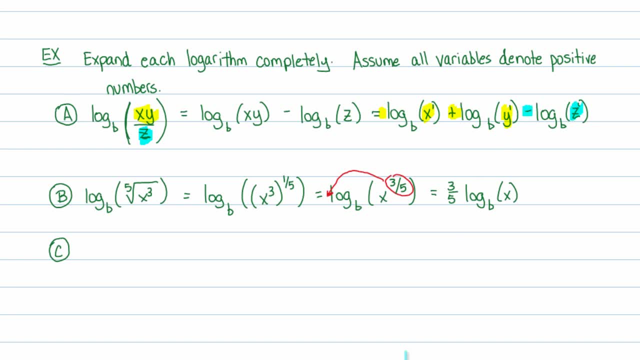 and the logarithm with Z in it was negative. So a great shortcut is to really notice. when you start splitting things apart, you just say, listen, okay, it's going to be like in this first example: log of X plus, log of Y minus, log of Z. 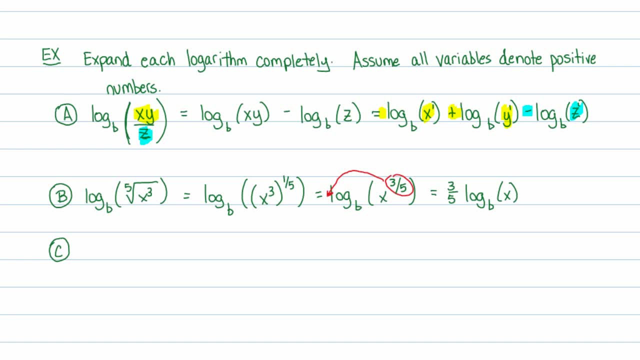 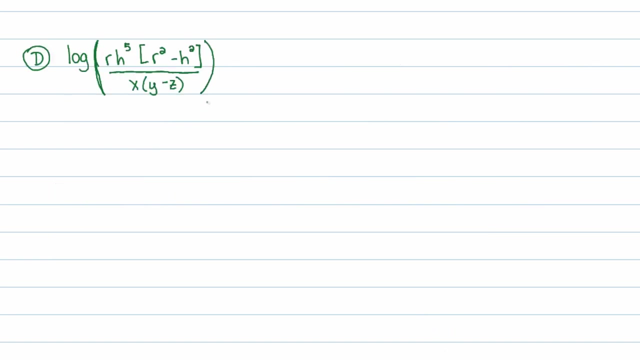 because everything downstairs will have a negative in it, Okay, Or a negative in front of it, in front of the logarithm. Notice: in the second example there was no denominator, So there were no subtractions in our final answer. So let's do one last expansion example. 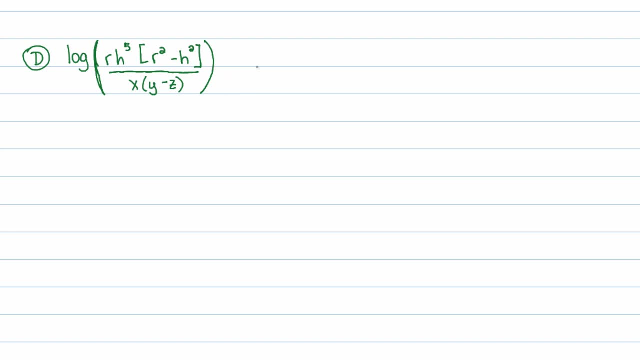 and this time we're going to take advantage of our newly found quick textbook, which is: everything in numerators splits into logarithms that are positive and everything in denominators splits into logarithms that are negative. First thing you want to do is focus on the inside of a logarithm. 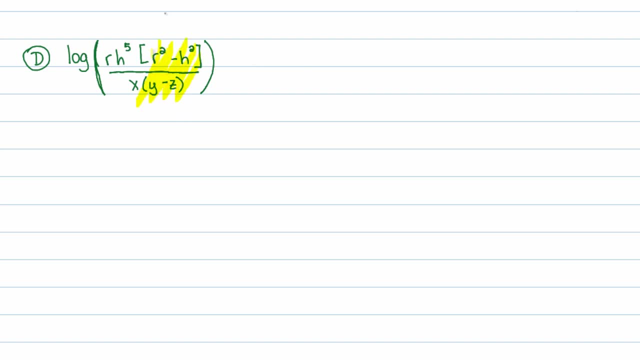 to see if you can clean anything up in here, And what I can see in there is there is something that does clean up. actually You might not see it. Like, for example, there are no R's that cancel between numerator and denominator. 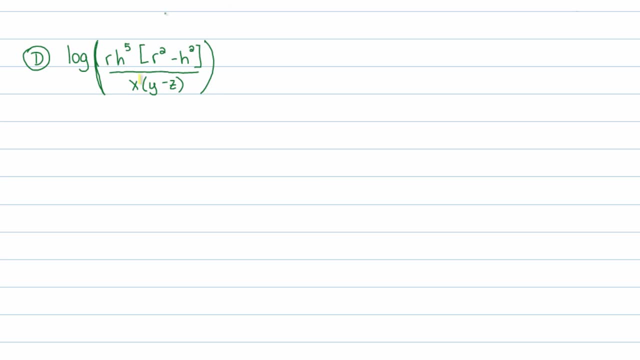 There are no H's either. I would not. I would not ever distribute that X through. You always want to keep things as factored as possible. But, that being said, if I want to keep things as factored as possible, see this bit right here. 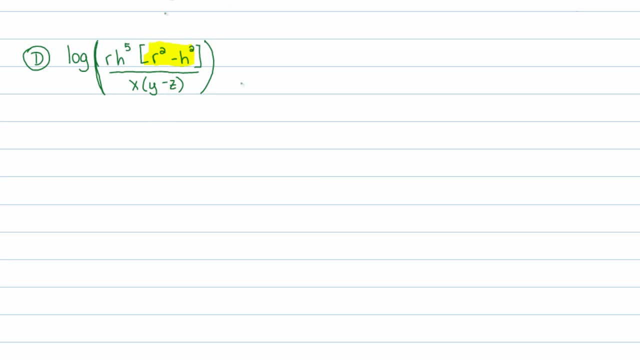 That's a difference of squares That can actually be factored. So I would first start by making sure the inside is completely factored. So that would be an R minus H times an R plus H. Super important to do that, It just really does make a difference. 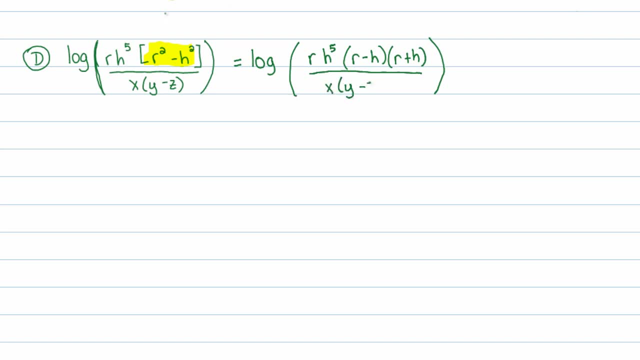 Okay. So always when you're doing these logarithmic expansions, make sure you factor the inside and cancel anything that you can first Beyond here. everything, all the each factor upstairs is going to end up as a positive logarithm, That is, you'll have a positive log of R plus log of H to the 5th. 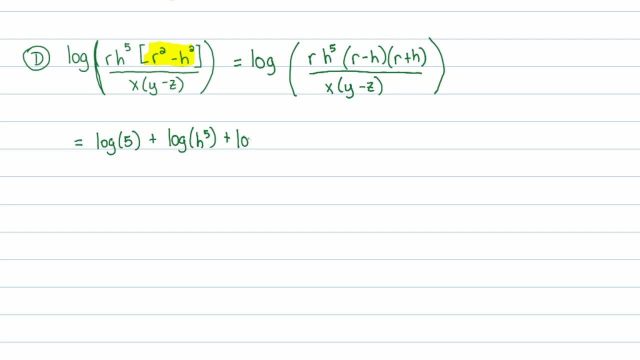 plus log of R minus H, plus log, plus log of log of r plus h. and then everything downstairs, which i'll go ahead and highlight right now. everything downstairs will have negatives in front of it. so minus log of x, minus log of y minus z. 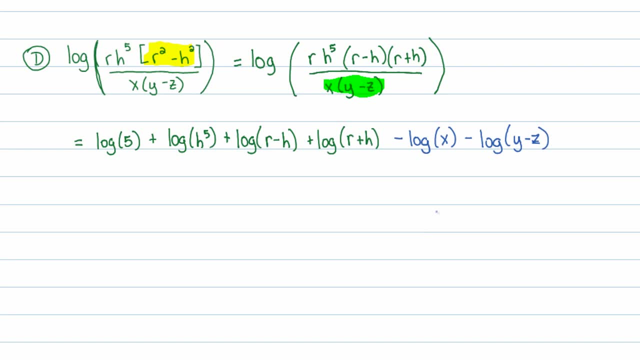 now we start looking through these to see if any of these can be simplified further. it turns out that one of them, and only one of them, can simplify further this one. right here, this power can be brought out front, and then, as i rewrite this, i'll tell you why. 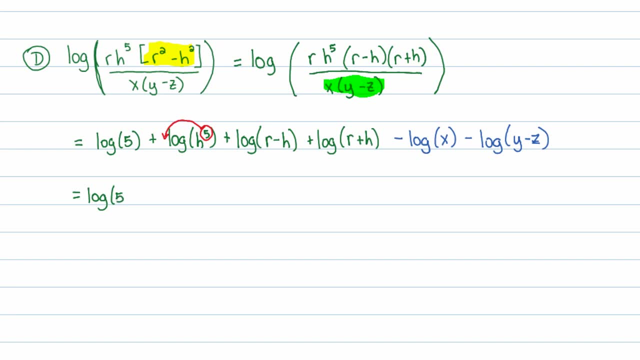 the other ones don't simplify. well, log of five doesn't simplify because it just doesn't. so five: log of h plus the second one or, i'm sorry, the third one, which is log of r minus h. if you look through our properties, we do not have one that says log of something plus something splits apart, right? none of these. 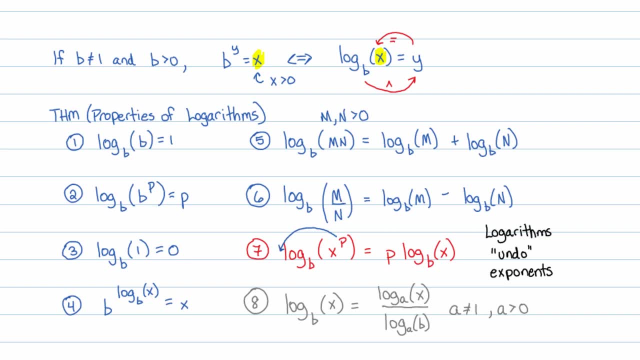 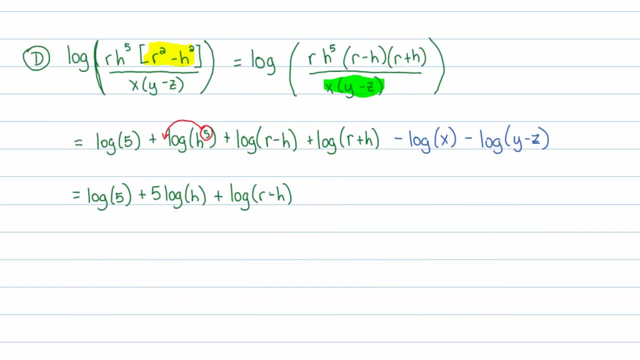 have a plus or minus inside the logarithm at all. you will never see a theorem like that. so do not think that you can split apart a addition or subtraction that occurs on the inside of a logarithm. if you have an addition or subtraction, you're stuck with that addition or subtraction. 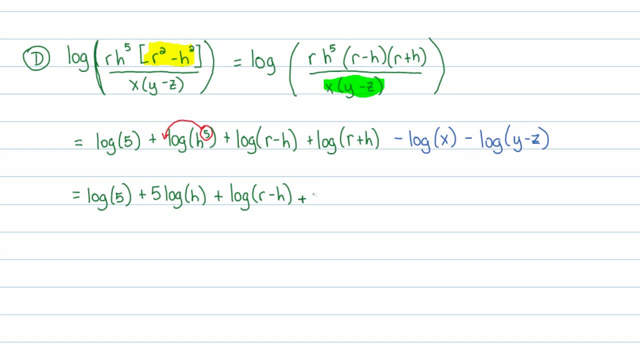 there's no other way to simplify it, it's just there. so everything left that i have additions or subtractions- is a plus or minus inside the logarithm. so if you have an addition or subtraction with, i just have to rewrite them. there's just nothing else i could do. 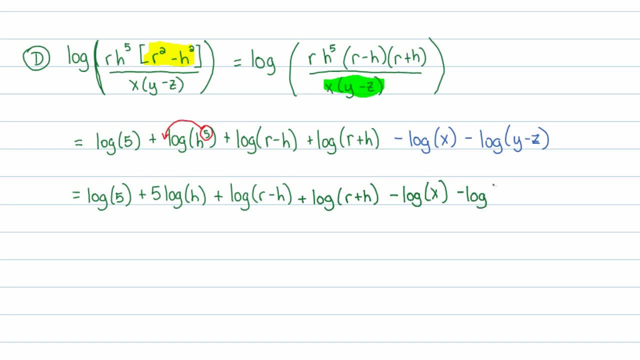 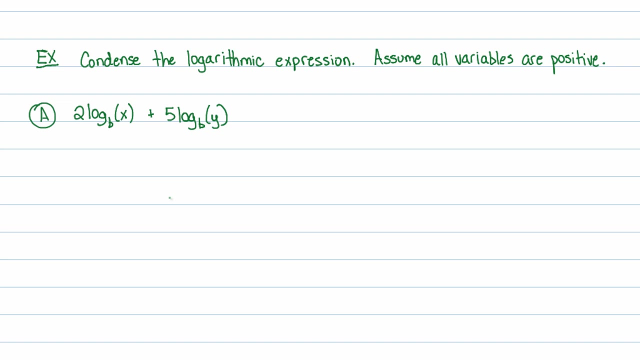 that right there is fully expanded. there's nothing that combines. and you can guarantee nothing combines if you just take the time to simplify your logarithm in the beginning. so now we've laid some great groundwork to work backwards, because working backwards is pretty fast once you understand how to. 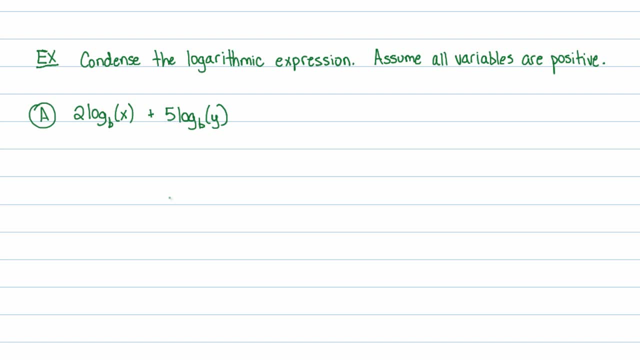 expand a logarithm. condensing the logarithm is pretty fast, so here we're asked to condense the logarithmic expression. assume all variables are positive. again, because inside a logarithm you must. the domain of a logarithm is basically positive numbers, so you must only insert. 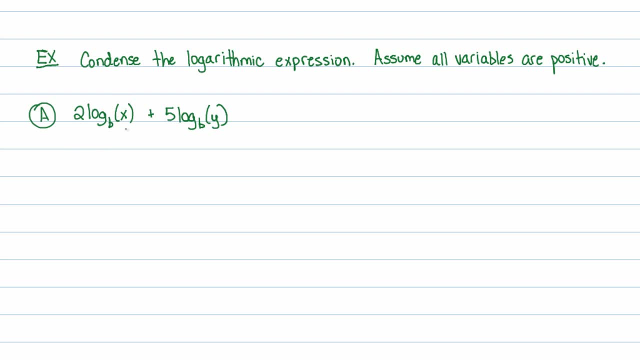 positive numbers into a logarithm. all right, first thing i'll do here is i look at this now. a lot of students start this problem and they just say, oh, that's like log of y, right, because you have a log base b of x plus log base b of y. it's not necessarily that if you 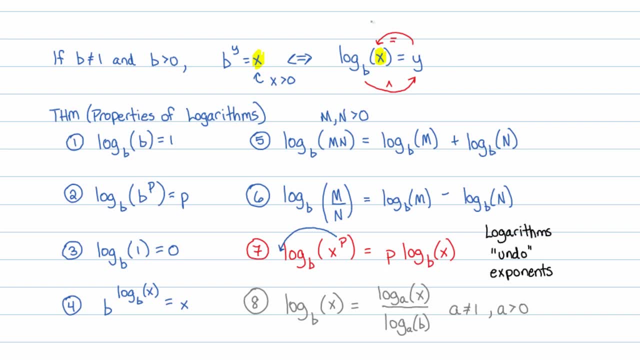 look at the theorem. the one i'm referring to is this one right here. if you have log base b of something plus log base b of something else, yes, you can combine it into one logarithm and it's the product of those two somethings. but it's not five times the log base b of m plus two times log. 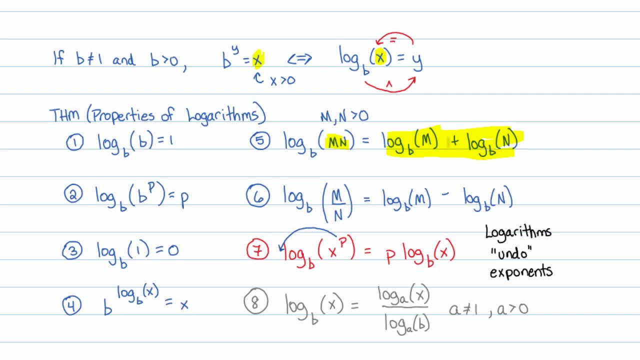 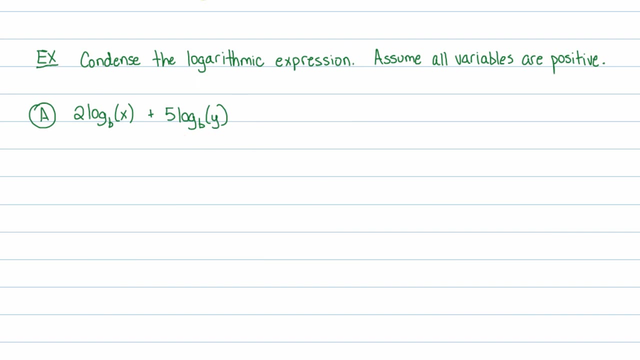 base b of n, it's a single log plus a single log. so we have to get these things, these logarithms, these things. we have to get these logarithms to have unit coefficients or- you lead- coefficients of one. so i'll do the opposite of our very special property here, this seventh property, instead of 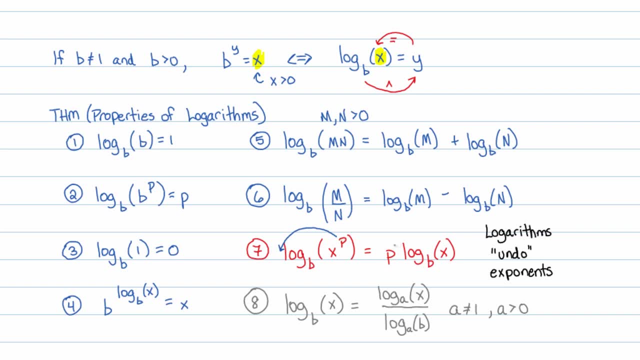 bringing the power down. i'm going to suppose that i start with a power out from this. i'm going to bring the power up to the x-axis, so let's go ahead and do that in our example here. i'm going to bring that two up to the exponent. 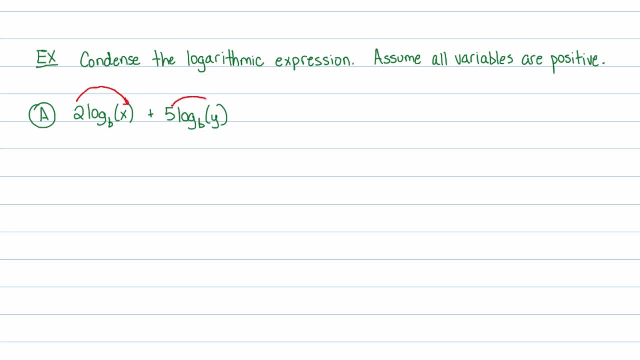 notice, i'm just going backwards, bringing this five up to the exponent in the y. if i do that i'll get log base b of x to the second power. so it's a single log base b of x to the second power plus a single log base b of y to the fifth power. 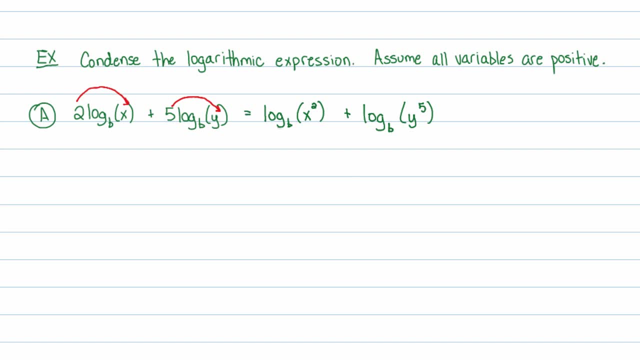 now that these are single logarithms with the same base- and it is required, by the way, that their bases be the same in order to use the theorem- we now know that these two can be re, or these two terms can be rewritten as a single term. log base b of the first input times the second input. 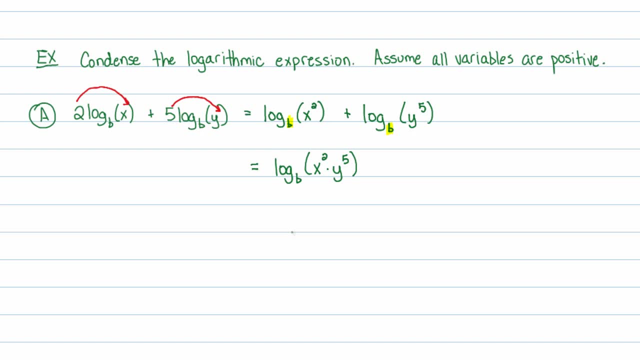 this is log base b of x squared times y to the fifth, that is completely condensed. that's all there is to it. there's. you can't go any further than that. so that's. that's as good as it gets. that's what you want, and when you condense a logarithm, by the way you want to make. 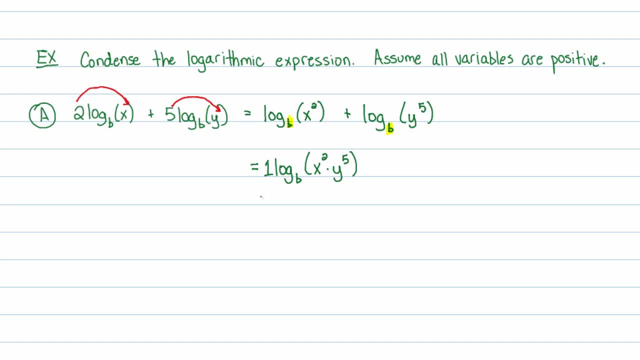 sure, your lead coefficient is one, and it is in this case. let's do another example. so here, in this case, i have a lot of action going on. i'm going to clean up things first. uh, for example, i'm going to distribute that negative two to each of those. uh, you don't have to do that. actually, you can. 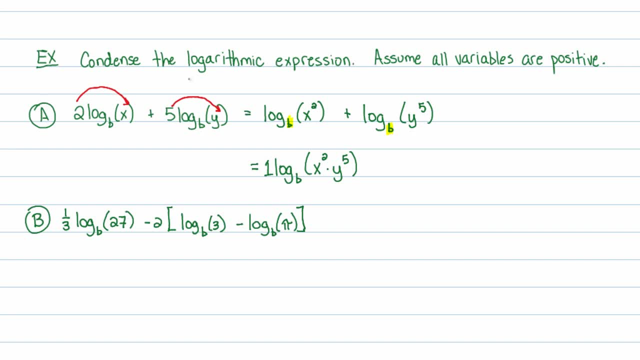 combine these first. in fact, maybe i should follow the order of operations. let's follow the order of operations. the order of operation says: focus on the inside of the innermost parentheses, which means on the inside of the each of these logarithms, if there's any addition, subtraction or anything like. 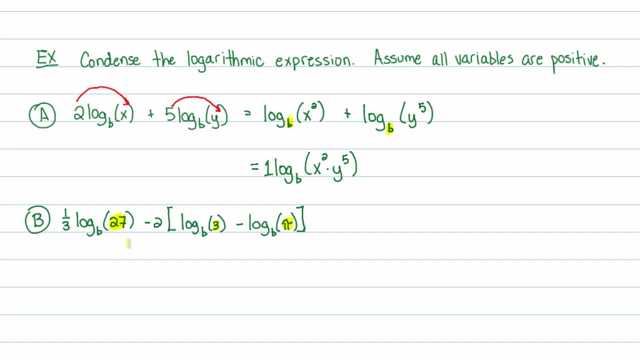 that on the insides, take care of them. but i'd look on the innermost parentheses. there there's no addition, subtraction, multiplication, nothing like that. so the next thing i do, again following the order of operations, is i focus in on the next outermost set of parentheses. 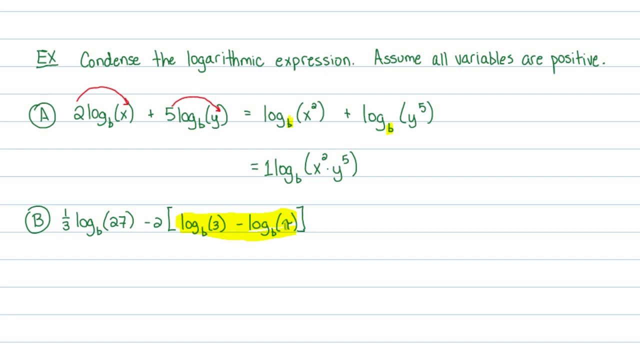 set of parentheses, which is these: this set right here, right, so i have log base b of 3 minus log base b of pi. okay, that means remember if one of them is positive and the other one's negative. that means the one that's positive will be in the numerator and the one that's negative will. 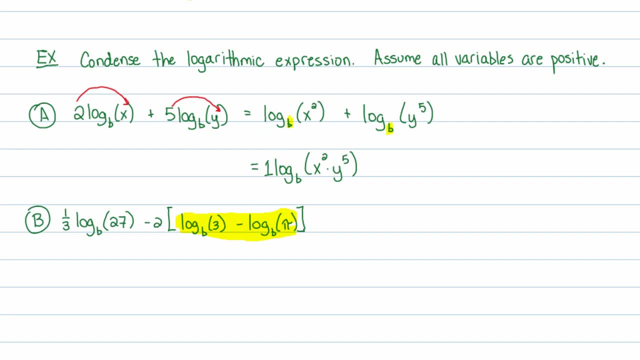 be in the denominator. so let's go ahead and do that. i rewrite the first thing because i'm only going to do a little bit of the time here. one-third log base b of 27 minus 2 times this will compress to log base b of: since it's a positive logarithm, that 3 will be in the numerator. 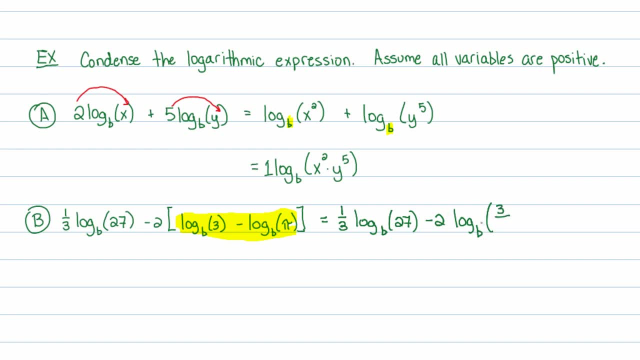 and negative logarithm, that pi will be in the denominator. so i already compressed this down right, just following the order of operations. now, again following the order of operations, you're going to do a little bit of the time here. one third log base b of 27 minus 2 times. 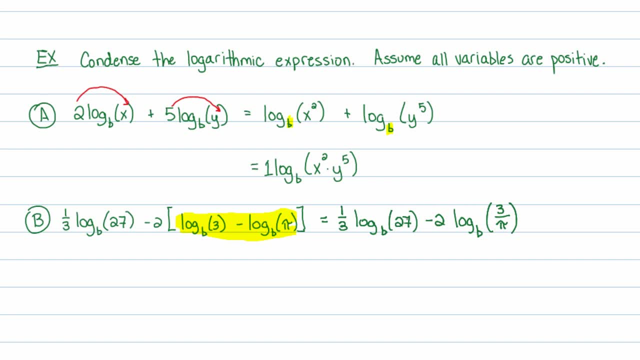 you look inside these parentheses again, 27 still doesn't simplify and 3 over pi really doesn't simplify to me. so now i look at each term and i'm going i start asking myself: is there any multiplication or division going on? and there is some multiplication. i have one third times the log. 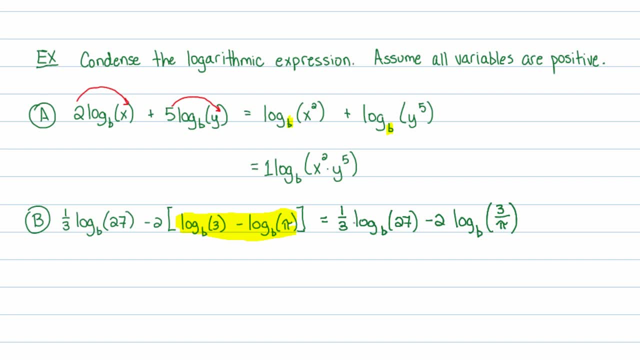 and two times the log, and i know what i could do with that one third and that two. i could pull them up into the exponents. so a two i'll pull up in this exponent as well. all right, do, uh, you're more than welcome to pull the negative two. by the way, some people ask: 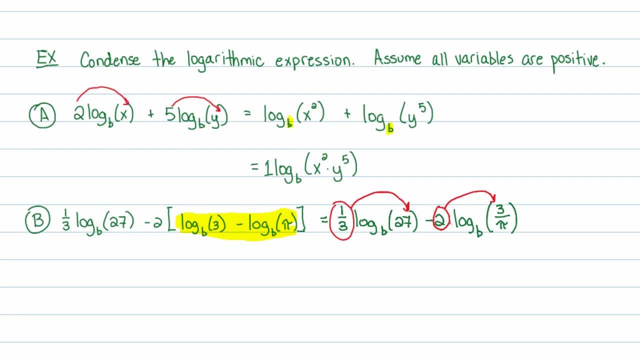 during my courses. can i pull the negative two up? well, you can, but it does get a little confusing for some people if they do that, because they pull the negative two up and they don't replace that negative two with a plus sign. so if you have a of a habit of missing negatives, which most of us do, 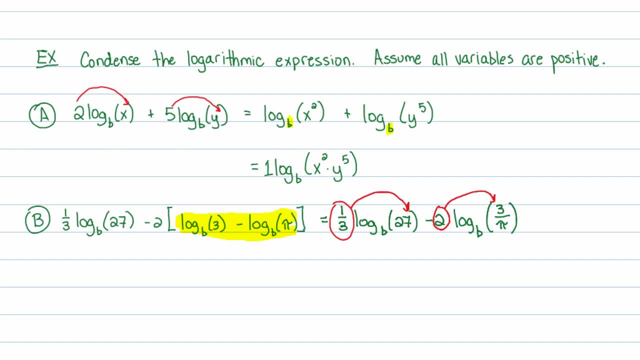 actually i'm going to do a little bit of that, so i'm going to do a little bit of that, and i'm going to do a little bit of that, and i'm going to do a little bit of that, and i'm going to request that you do not steal the, the minus sign. just take the two and put it up in the in the. 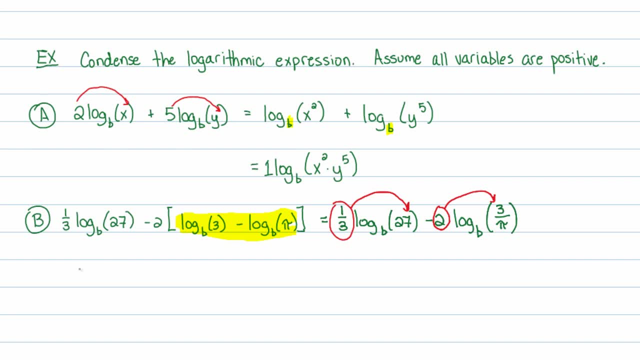 numerator. so we get this or up in the exponent. i'm sorry, we get this log base b of 27 to the one third power, minus log base b of three over pi being raised to the second power, and again follow the order of operations in her most parentheses. so inside this: 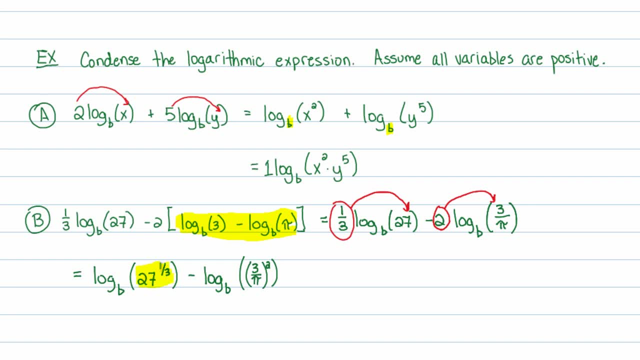 parentheses. I see I can actually now do something. I've all of a sudden created work on the inside of a parentheses. I could take the cube root of 27 pretty easily. that's just 3 and over here I can actually apply this square as well. so I 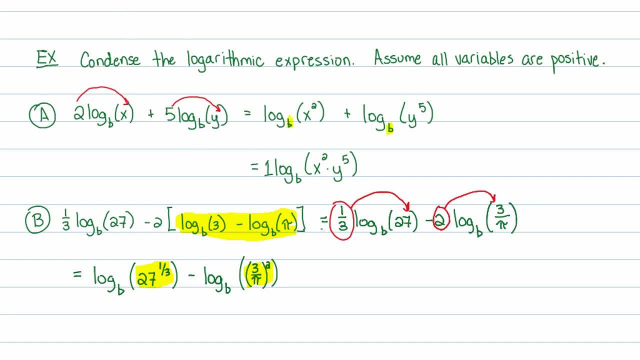 could clean this up a little bit before I go any further. this is going to be log base B of 3 minus log base B of 9 over pi. Oh, 9 over pi squared. somebody was likely about to type something to me. yeah right, it's, the square affects both. 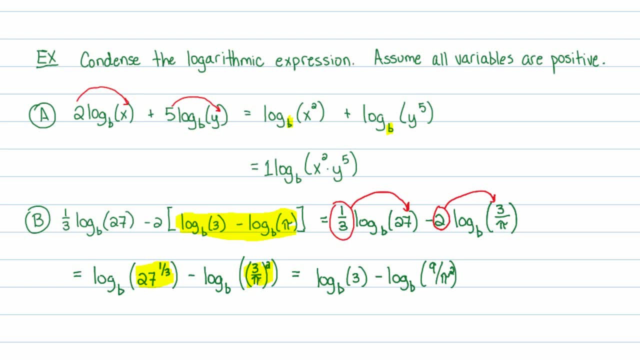 the 3 and the pi, so it's 9 over pi squared. there we go. almost mess that up. at this point I'm going to go ahead and again do one last little check on the inside. you again following the order of operations. is there anything to do on the inside? the answer is no. both these: 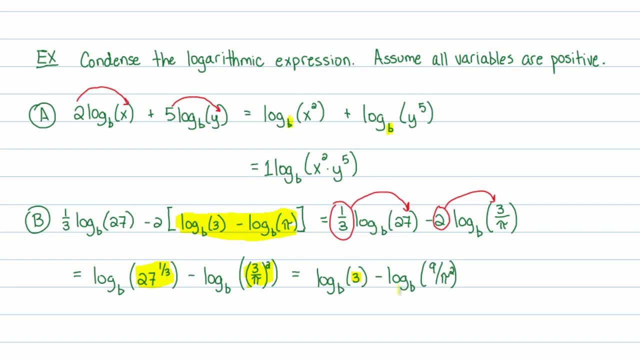 parentheses. on the inside, there's nothing to do. so now again, I focus on the outside, the parentheses. well, I asked myself: is there anything multiplying this? no, anything multiplying that? no. is there any addition or subtraction? sure, there's a subtraction right here, and I know I have a theorem. theorem for: 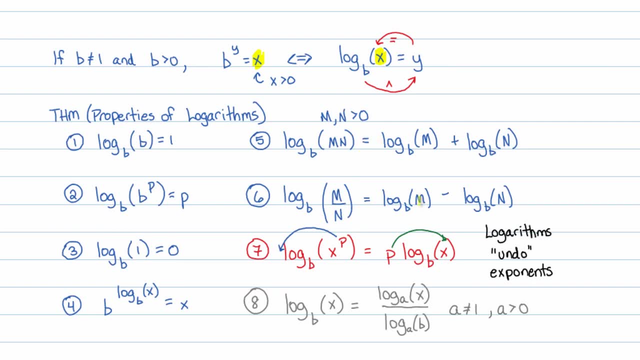 subtraction. right. we have this log base B of something minus. log base B of something else can be compressed into a set of elements and I can have a set of elements and I can have a set of elements. single logarithm of the ratio of the two right: the positive stays on top the negative logarithm. 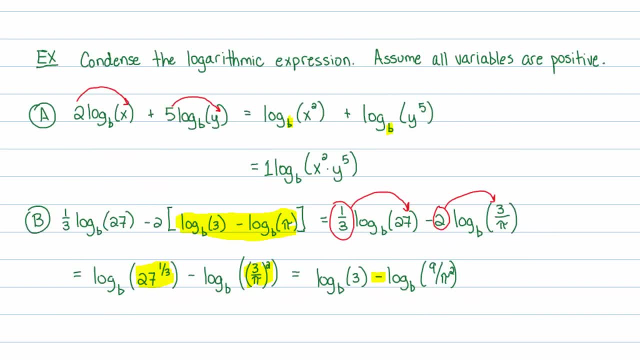 stays on the bottom. so let's go ahead and try that in this case- and there will be a little extra work at the end here- we'll have to do so. this is going to be equal to log base b of the positive logarithm, its input goes upstairs. the negative logarithm, its input goes downstairs. so i have a nine over. 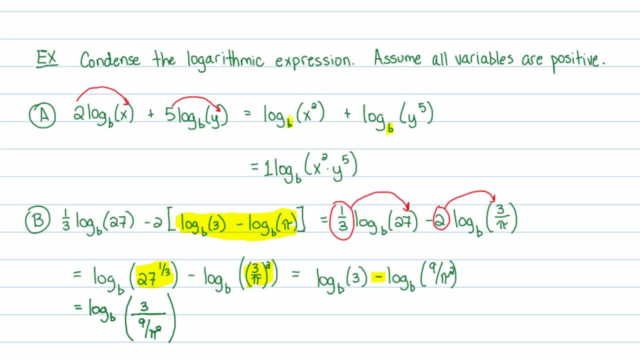 pi squared, which is kind of the funny thing here. so remember that if you have a situation like this, this is called a complex fraction. you never want to leave your answers as a complex fraction, so there's a couple ways you can think about it. depends on who's taught you. one student might. 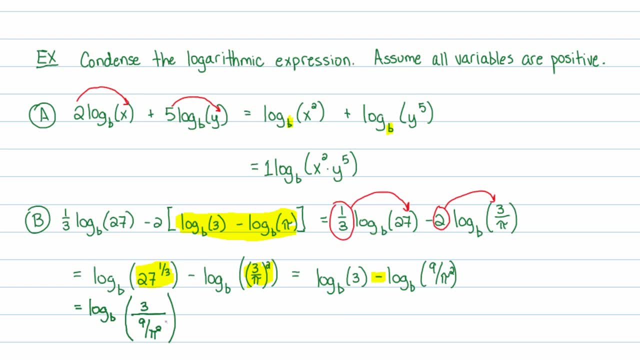 have been taught by somebody who says: oh, multiply top and bottom by the lcd, which would be pi squared, so multiply top and bottom by the pi squareds, they'll cancel and you will get the log base b of three, three pi squared over nine. course i, uh, i actually. 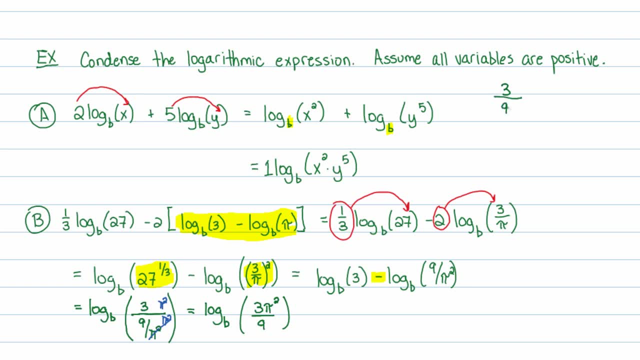 like to think of it this way: if you have three over nine, over something, nine acts as the hinge and the pi squared will just flip up the top, so you'll have a three pi squared over nine. in either case, you get the same answer. that's kind of the way i've always thought about it since i was a student. 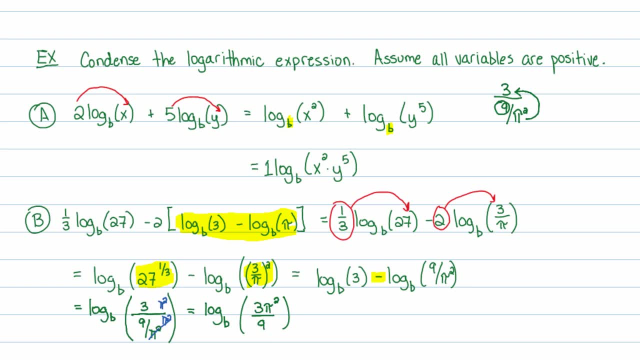 now, before we finish, you have to just make sure that you have cleaned your answer up as much as possible. it is a single logarithm, base b, but i see on the inside i can cancel a little bit. so clear this out: three goes into nine, three times. 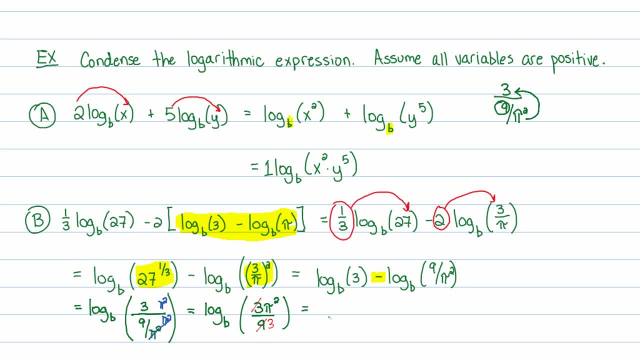 and so, finally, i have a nice, clean final answer of a log base b of pi squared over three. All right, that about does it for the theorems and the properties dealing with logarithms and expanding and condensing logarithms. In the next lecture I'm going to talk about more properties of logarithms. 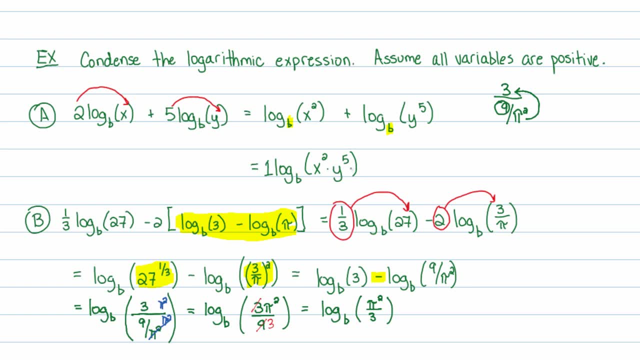 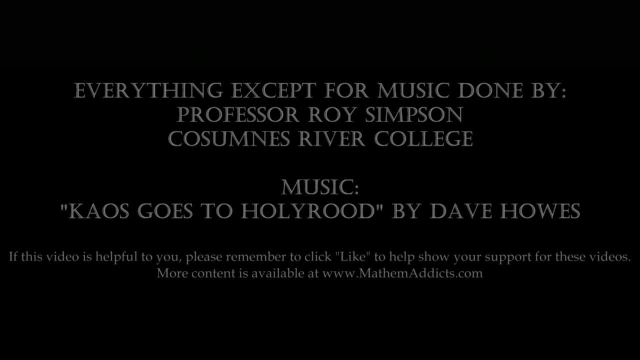 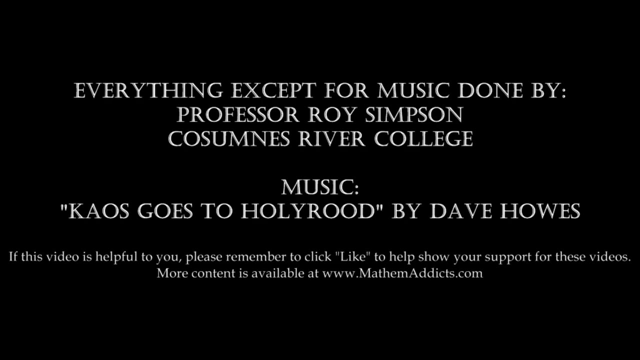 Well, maybe not more properties, but using the properties of logarithms to solve exponential and logarithmic equations. Thank you.